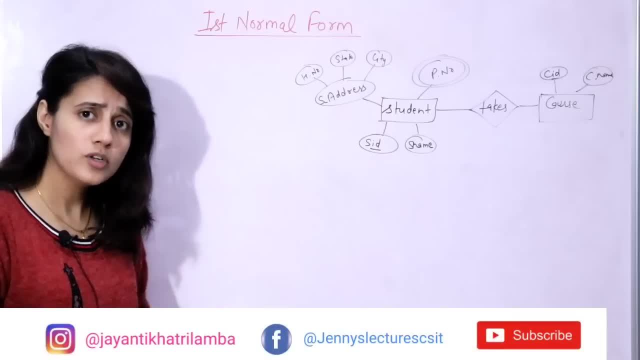 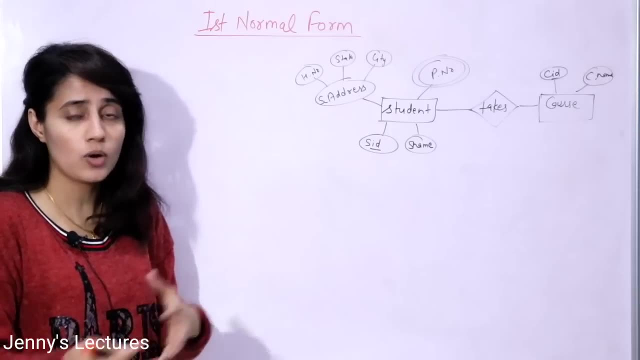 small er diagram. i want to show you fine now, once you when, when you convert this er diagram into tables or into relations. obviously you have to convert, you have to make a database, you have to design your database right. so you have to make some tables, you have to convert this er diagram. 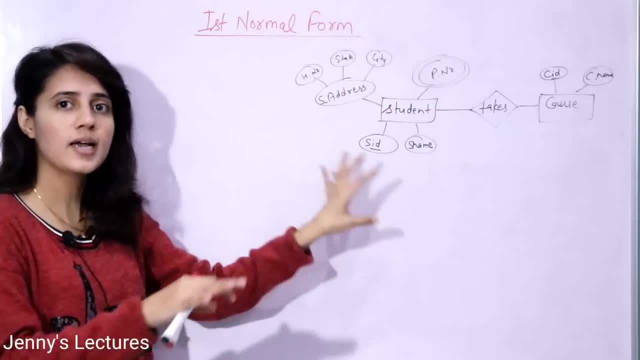 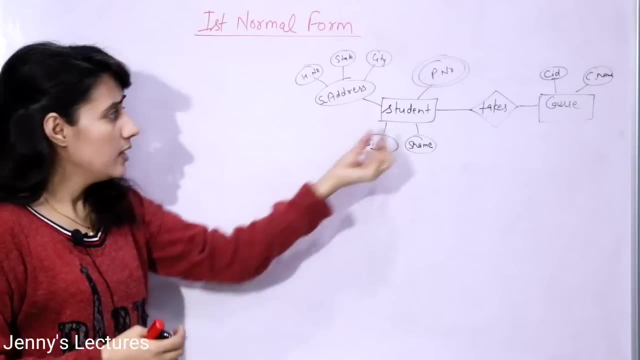 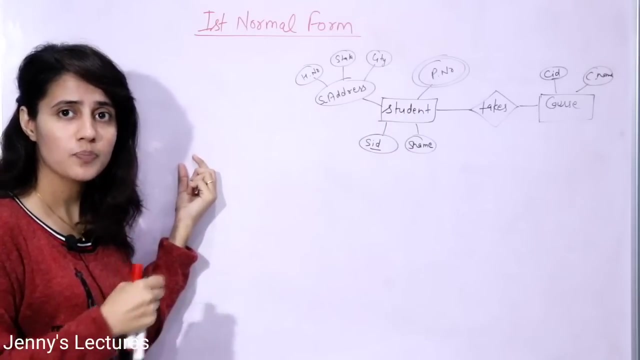 into relational tables- relational schema. how to convert er diagram into relational schema, that also we will discuss in a separate video. fine, so in that case in the table each entity is, you will consider as a table, table name is student and in that table attributes would be all the attributes of this entity right now, er diagram. 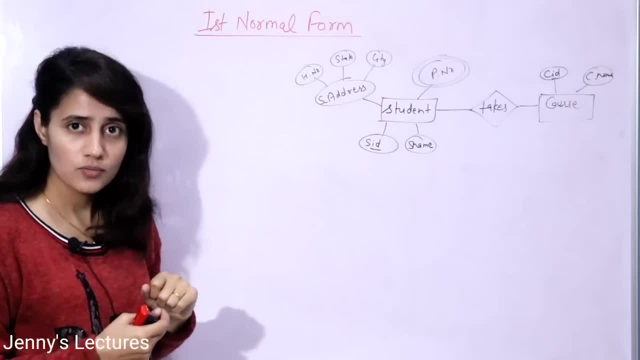 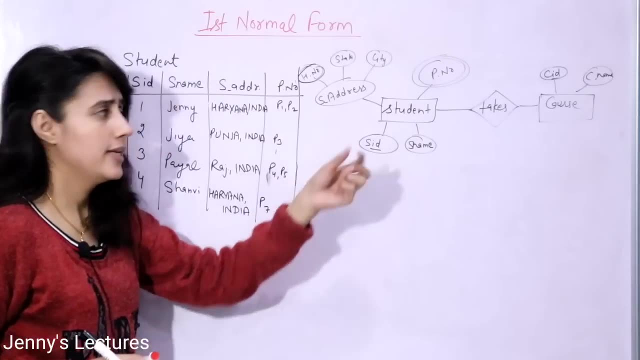 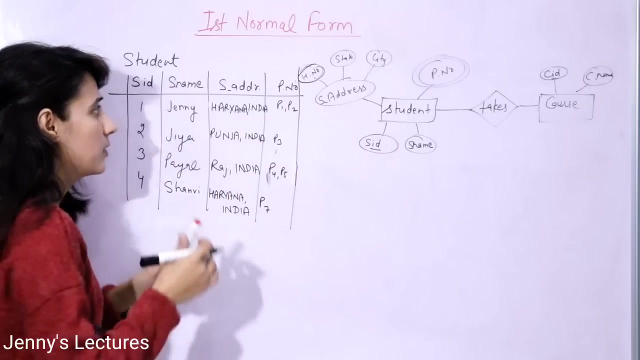 is having composite attribute as well as multi-valued attribute. fine, it means when you create a table, something like this: now suppose i have converted this, i have just taken only one entity, that is, student, and i have make only one table. not i'm going to complete the comp, going to convert the complete er diagram, right. so now here, suppose i. 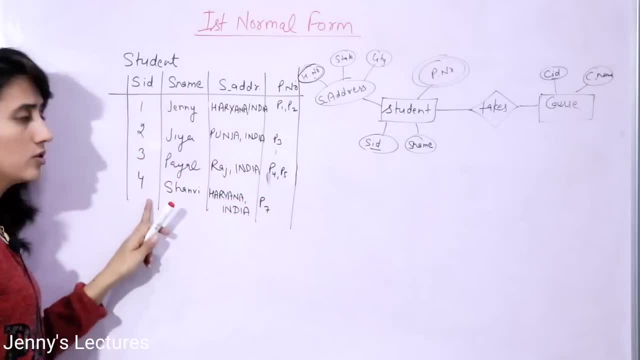 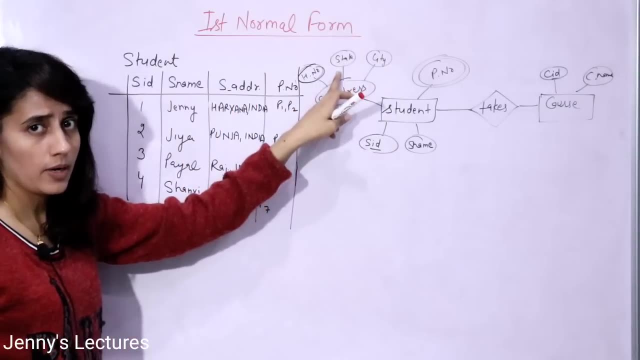 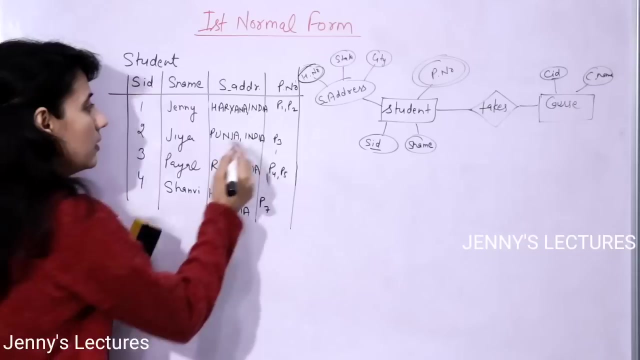 have written something like this: student id is primary key, so this is student id, right? student name, student address. in address i'm taking- suppose not taking all the attributes here- that is, house number, state, city. i'm writing only state and country. haryana, india. this is also punjab, you can. 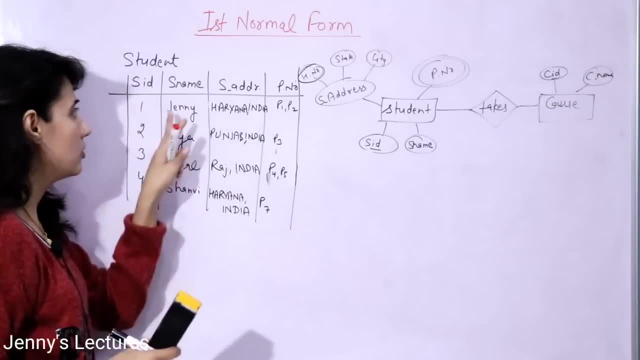 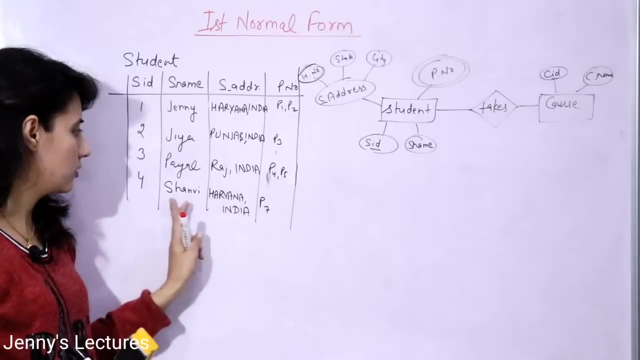 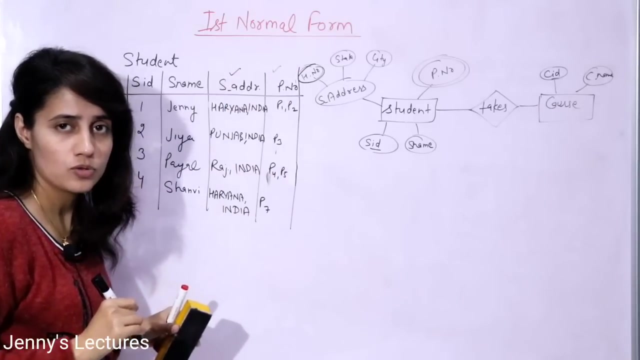 say india, rajasthan, india and haryana, india. and phone number are suppose this one, jenny is having this, is having, gi is having only one pile is having two and shanmi is having only one phone number. right? so this is what multi-valued attribute and this is what composite attributes. 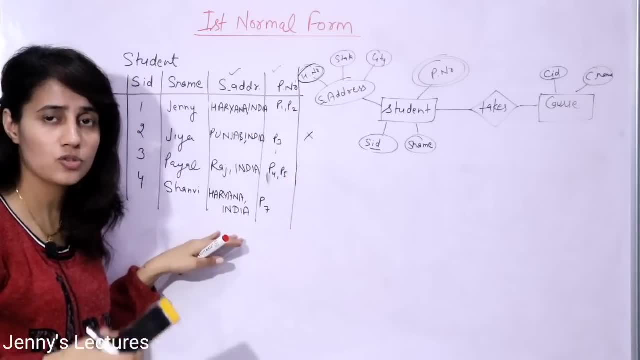 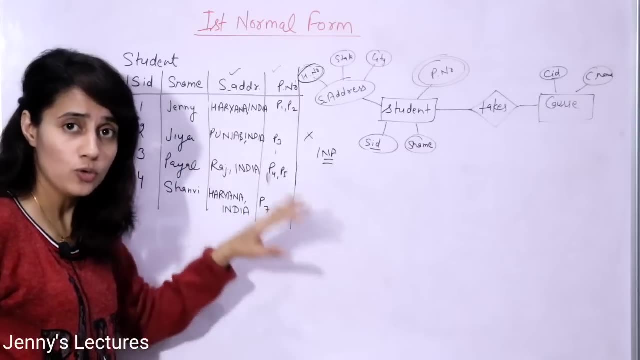 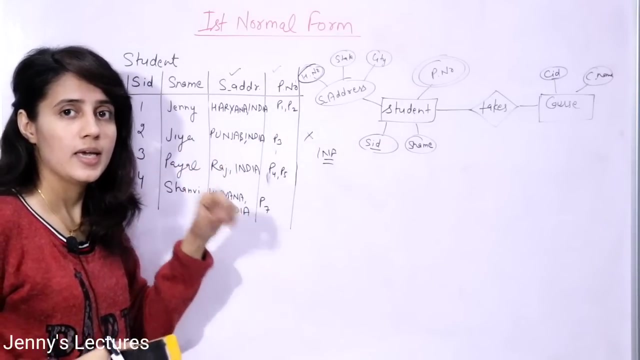 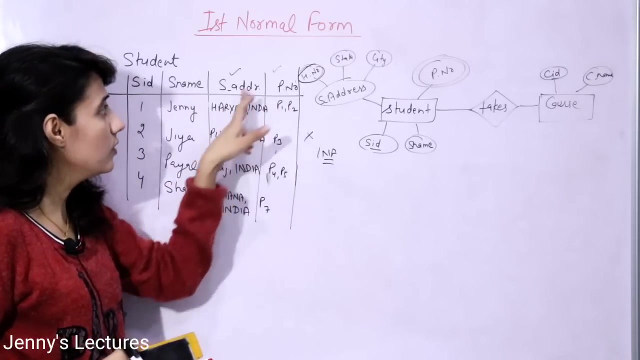 but this relation, this relational schema, is not in first normal form. you cannot convert it something like this. you cannot. when you convert an er diagram into relational schema, then relational schema must not contain any multi-valued attribute, right and composite attribute as well. now, if obviously, we will write: 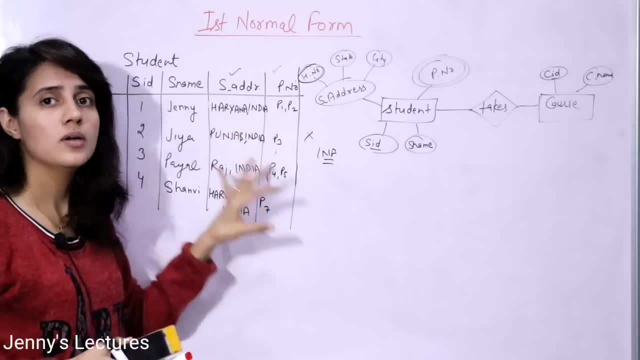 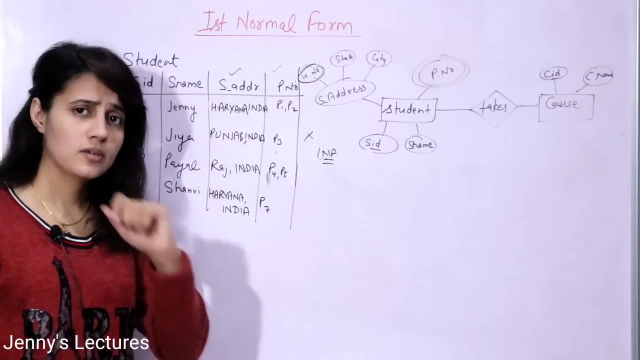 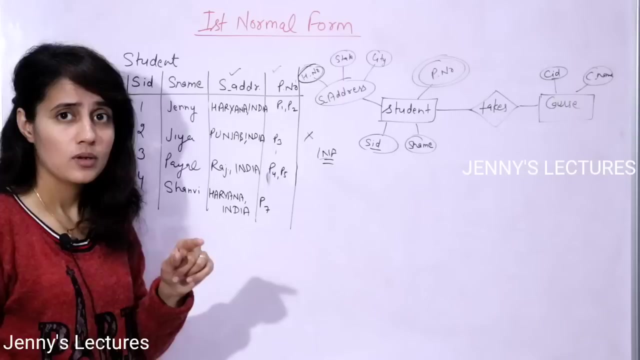 address and phone number here, but you have to convert it into now, first normal form. why this schema is not in first normal form? because the condition or the rule is: what a relation is in first normal form if, and only if, all the attributes are having atomic domains. 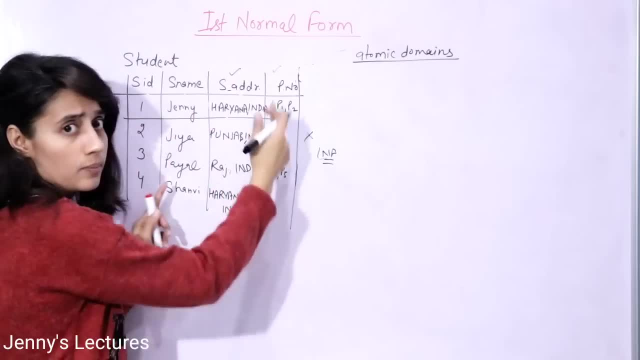 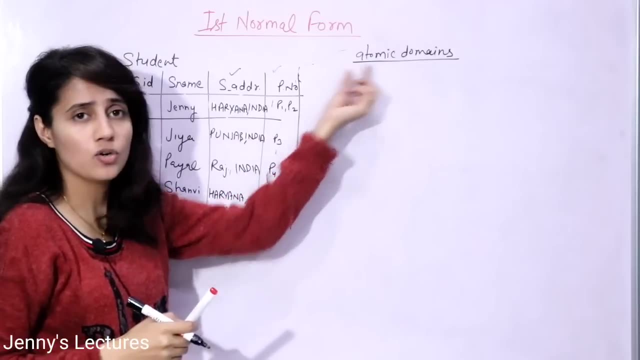 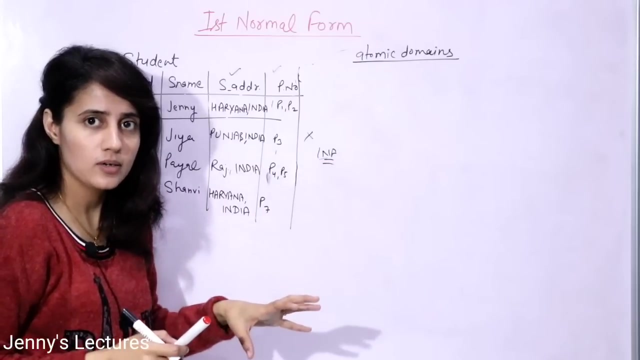 then you can say each column or each attribute- obviously this is what attribute. or you can say column. each column should contain atomic values. now, what does this atomic means? atomic means that cannot be further decomposed into smaller pieces by the dbms right. or you can say individual unit. 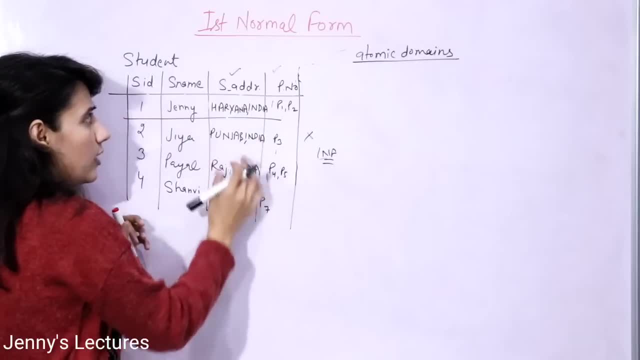 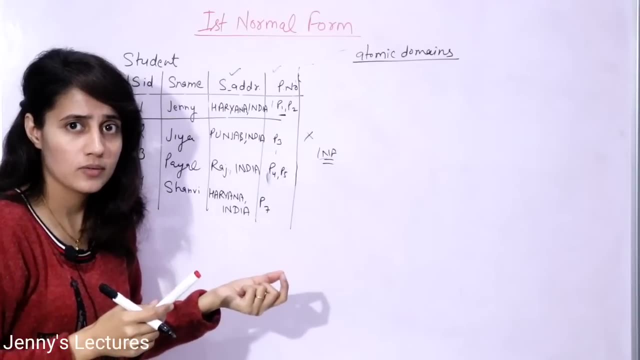 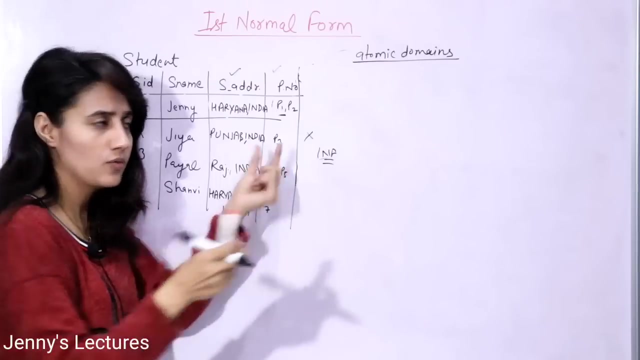 that is what atomic now, each cell, or you can say each column, but this column see what about this? p1 and p2, this is containing two values. it is not atomic, right? if this is what atomic, it contains only one value, that is p3. only one phone number, right? obviously there would be some phone number. 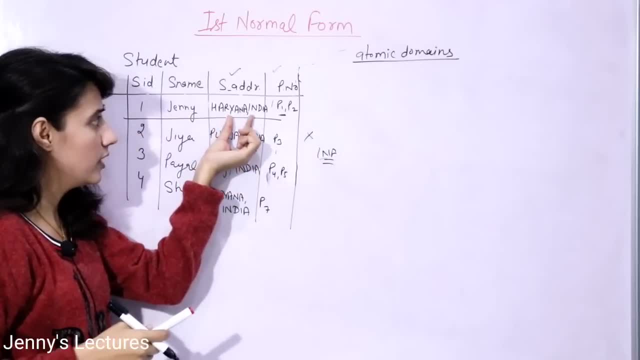 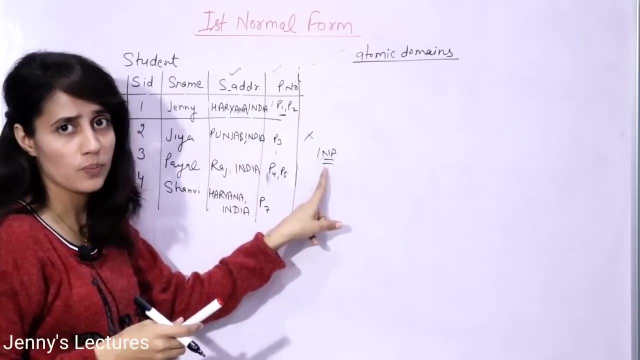 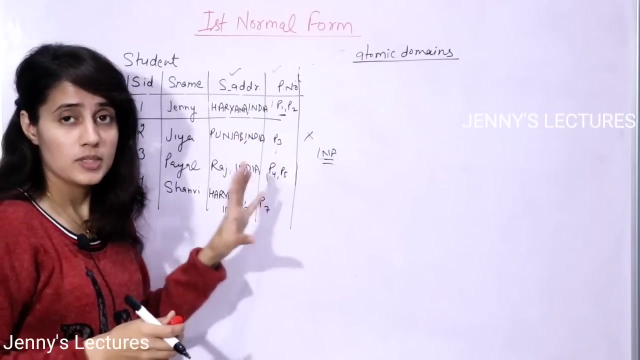 this is also containing two, so this is not atomic. this is also containing two values, so this is not atomic. so that is why this table is not in first normal form. if you want to convert it into first normal form, then you have to make each cell. atomic means each. 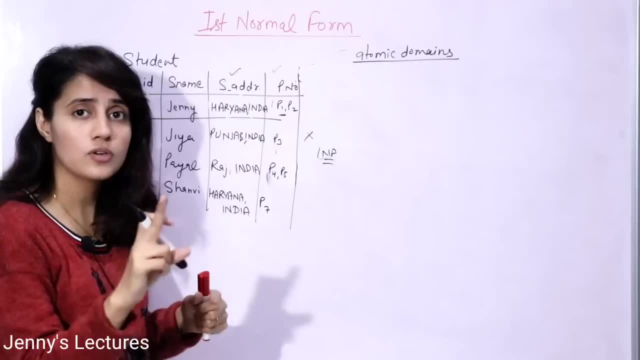 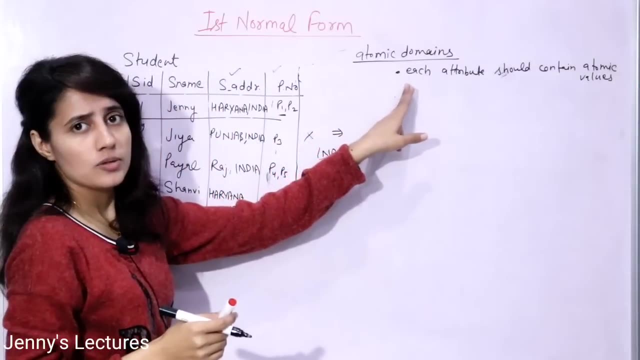 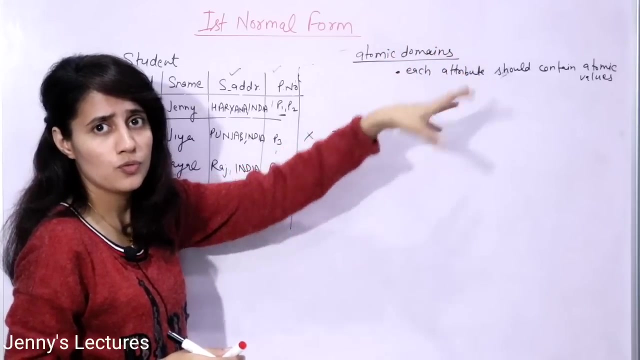 cell or each column should contain atomic values. right, that is the first rule and the very important, or you can say the main rule of first normal form. so this is the first point that each attribute means, or you can say the rules here you can write: a relation is in first normal form if it 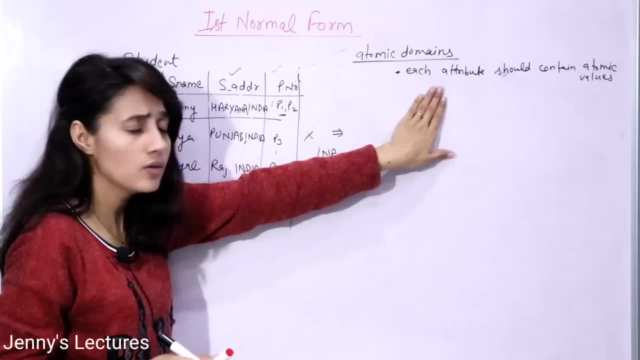 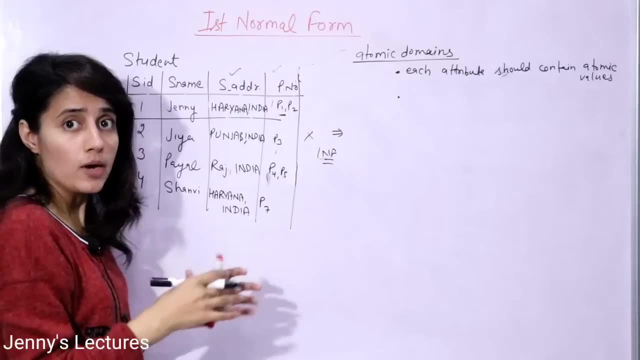 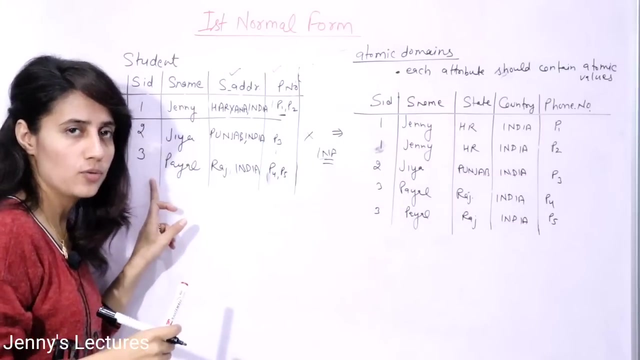 follows the following rules. and the first rule is: each attribute should contain atomic values. or here, in another word, you can write: each cell contains exactly one value, simple terms. now how to convert it into first normal form. see, suppose here I am taking only three student information, not four student information. so now how? 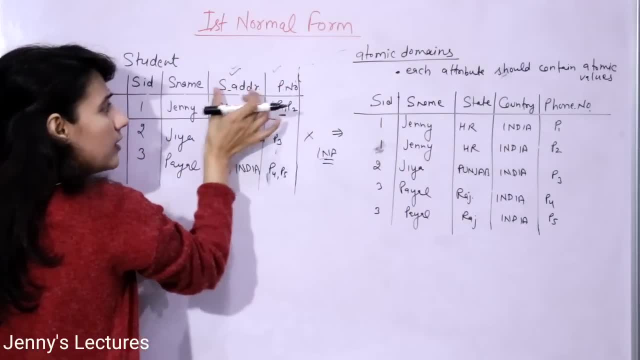 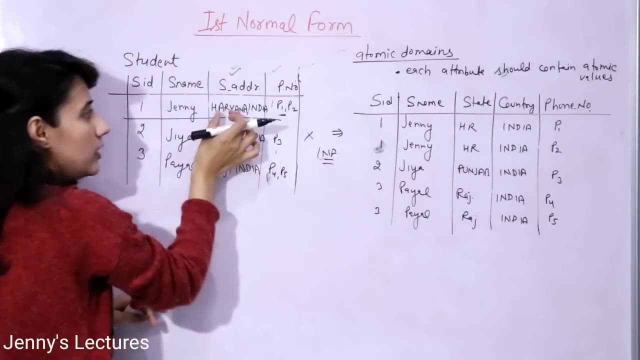 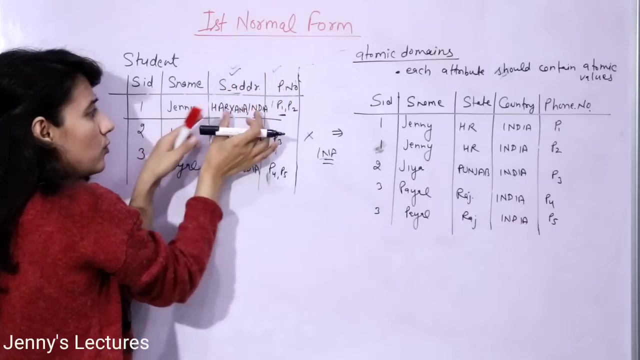 to convert it into first normal form. see, if composite attribute is there, then what you will do: you will make separate attributes or separate column for each of the attribute. so here is what in this composite attribute. this is made up of two attributes I am taking: one is what state, one is what country, so two: 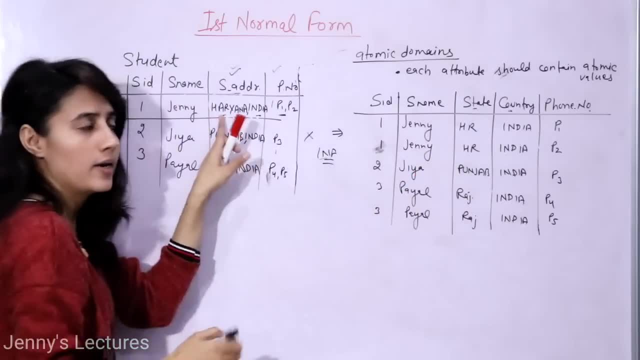 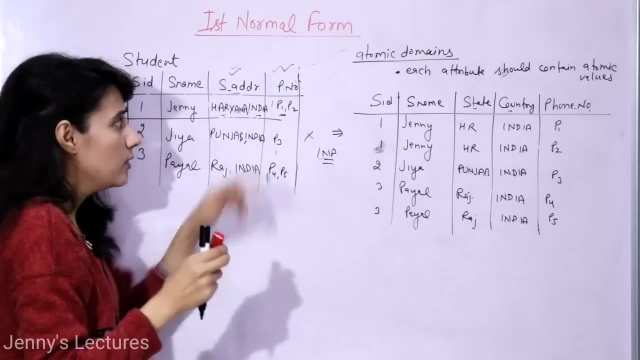 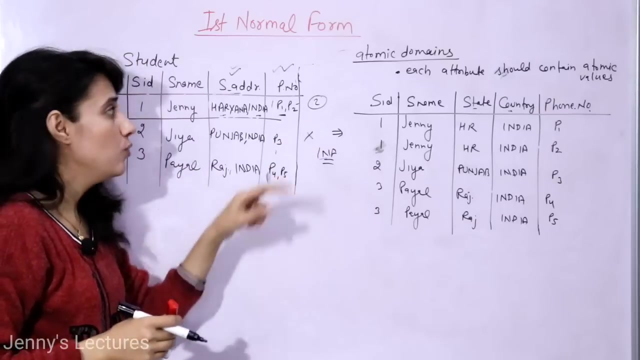 separate column you will make. one is for state, one is for country, and there you will write state and in one you will write India or you can say the country, right? what about multi-valued attribute? if multi-valued attribute is there in this multi-valued set, we are having two entries, right? so you will make separate. 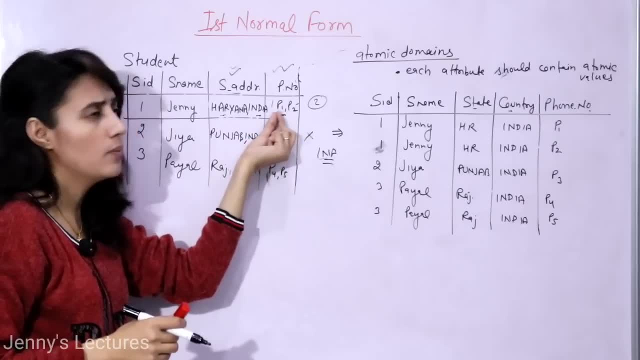 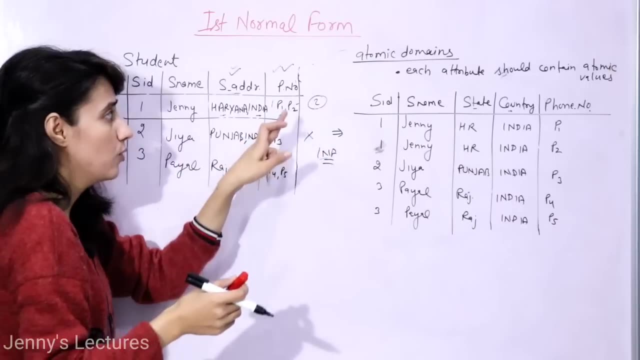 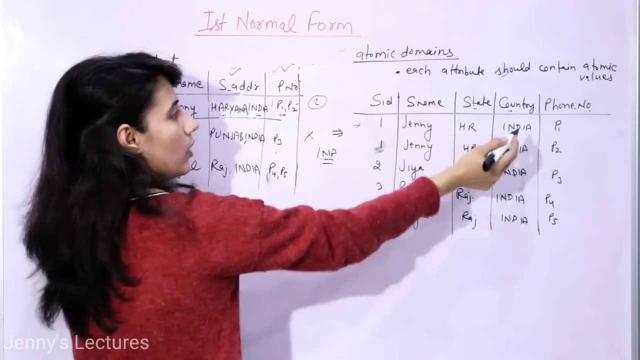 or you can say one tuple for each value in the multi-valued set. in the set I have two entries, so I'll you have to make two tuples, one for p1, one for p2. so in first tuple I am taking this one, Jenny, the address, and p1 in another. 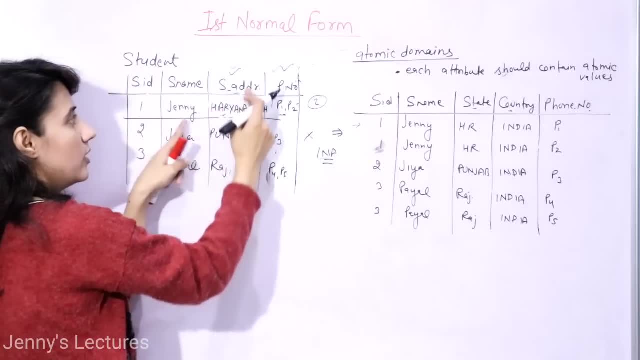 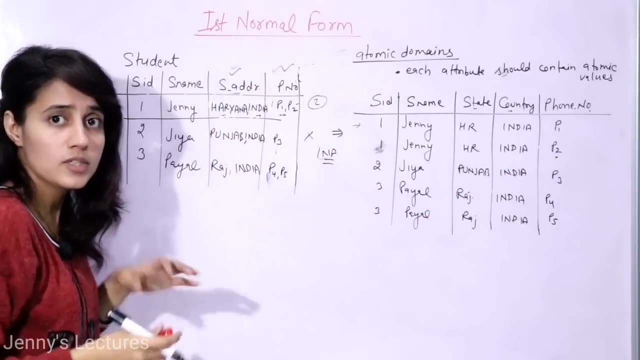 tuple again. obviously SID would be same, name would be same, Jenny address would be same. but only change is what? this one here we have p2. this is how we are going to convert it into first normal form. now you can say: this table is now in first. 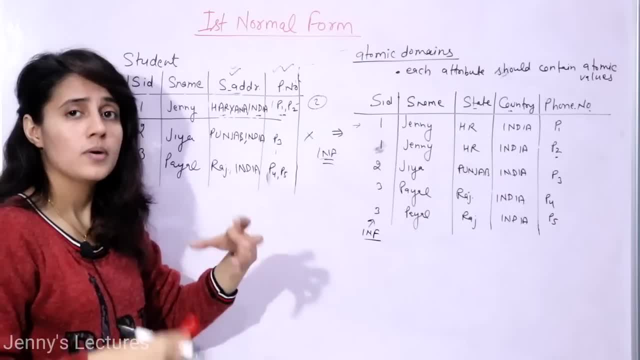 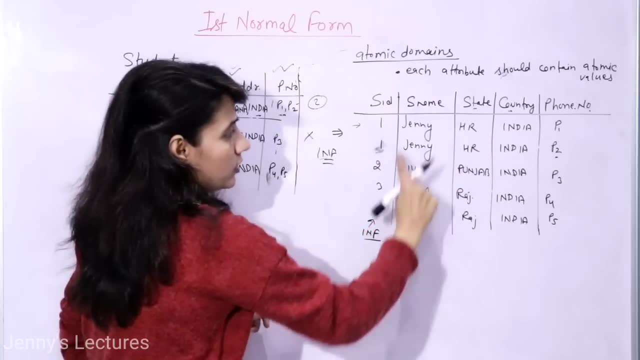 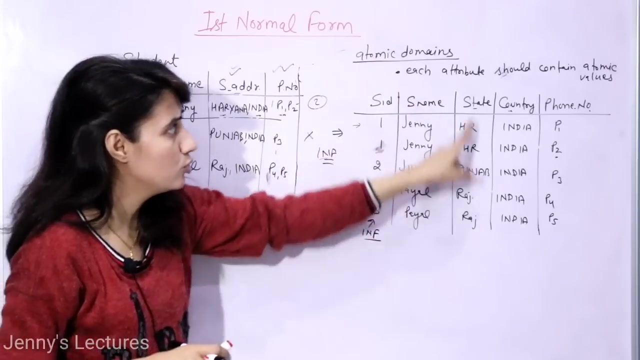 normal form, right. obviously we are having some another rules also here. we have discussed only one rule, right. I'm also going to discuss all the rules. see now, you can say each cell is having only one value. you can say you can see here, right. but you can say each attribute should is containing only atomic values- here, right. 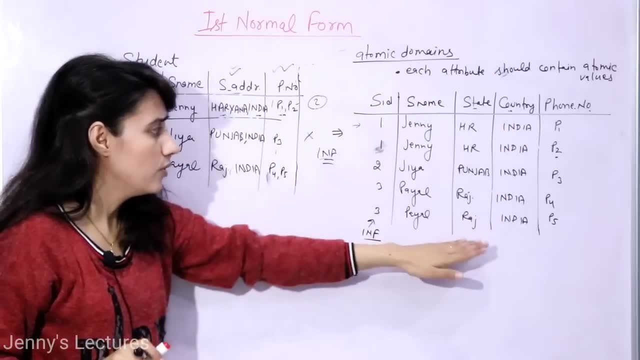 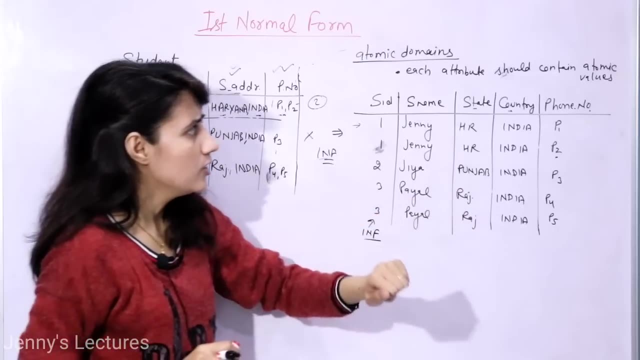 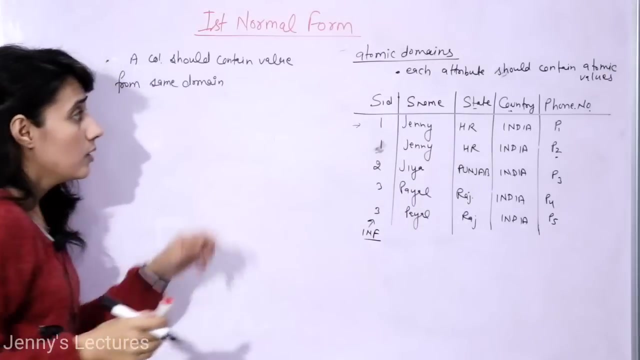 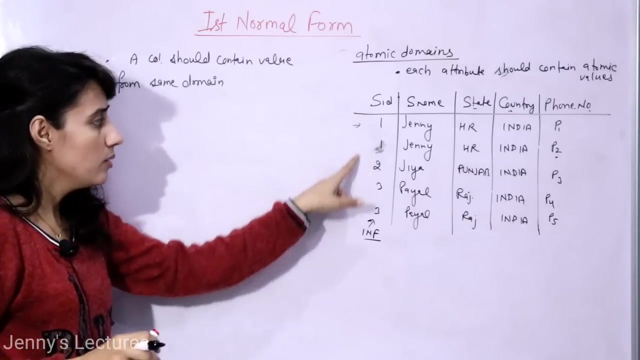 see, I'm not saying that this is the only way to convert it into first normal form. there are only mainly three ways. that also we will discuss right now. second point is: what second rule is? what first rule is this one? now? second rule is: a column should contain values from same domain. or you can say in simple terms, you can say a: 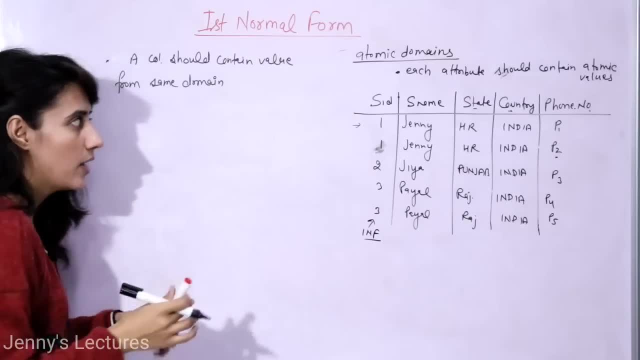 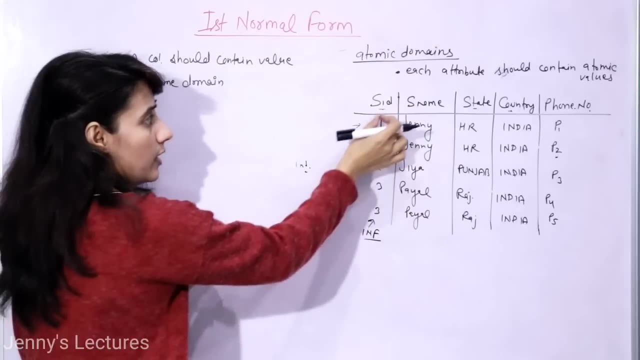 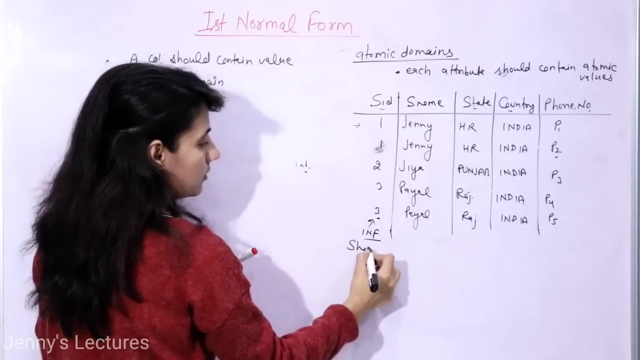 column should contain values that are of same type. now, what does that mean? SID? here I am taking this domain is what I am taking in teasers, right? so here we cannot store, we cannot here add S name like I'm. here I'm writing Shanvi and here I'm writing the row number four. that is wrong if you are this. 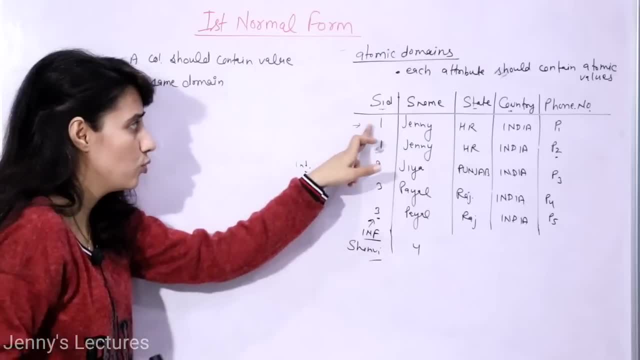 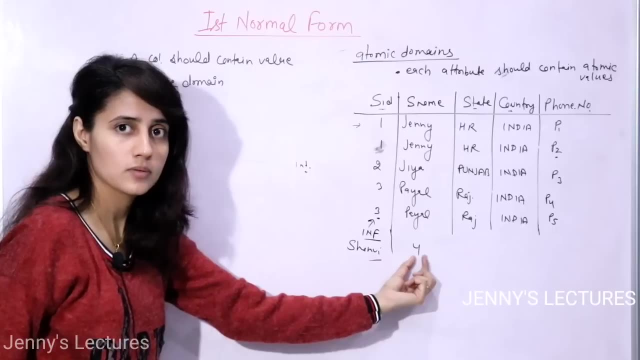 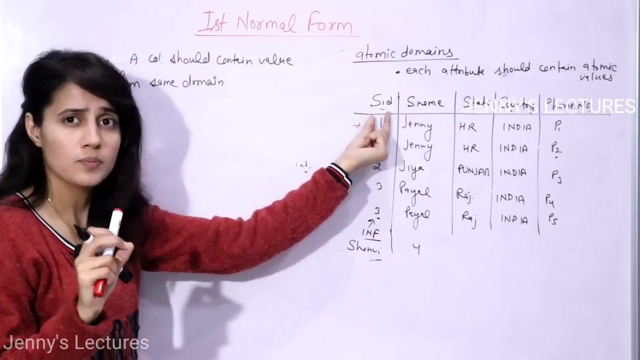 domain is what integer you are storing here the SIDs, then you will store SIDs only in every row. here you will store only S names. you cannot store all numbers right. so every column, the column, the domain is what? whatever the applicable domain on that column, all the values in that column should. 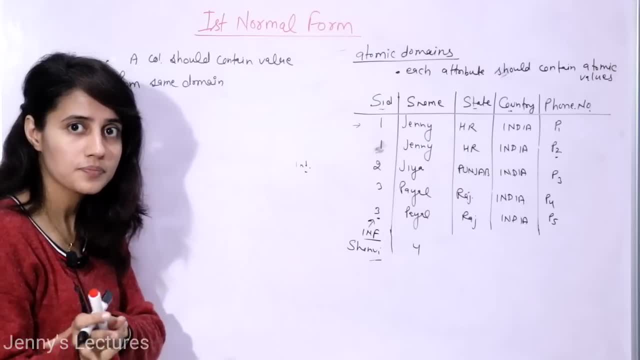 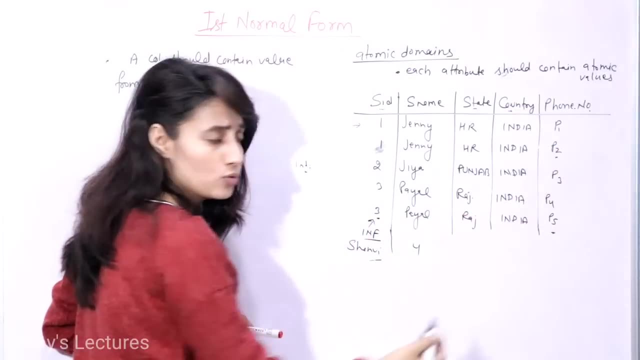 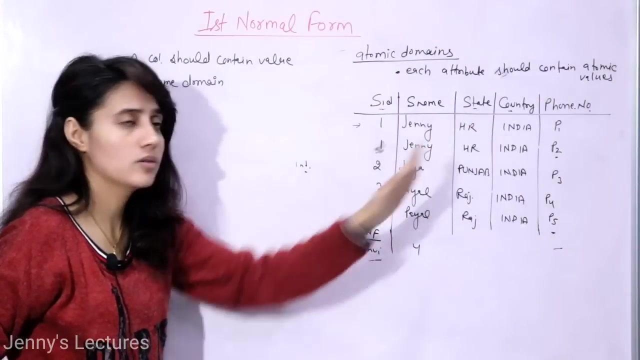 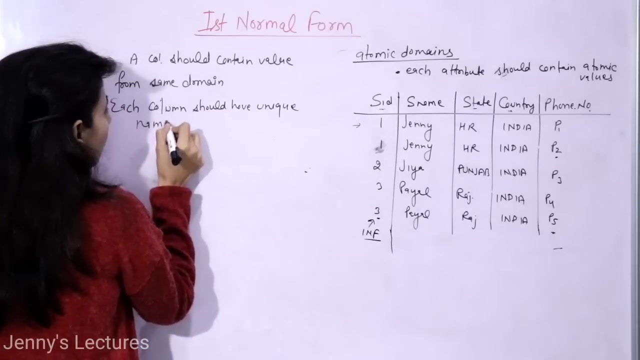 be from that domain only, right. here we cannot store integers value. here, obviously this is what integer phone number would be in integer form. so here we cannot store string values, right, because we have defined already the domain of each attribute, right? this is the second point. now third rule is what each column should. 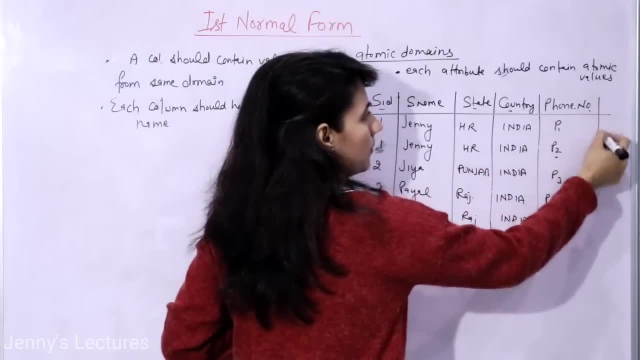 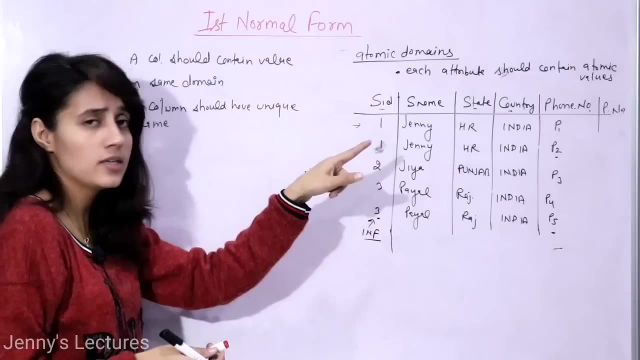 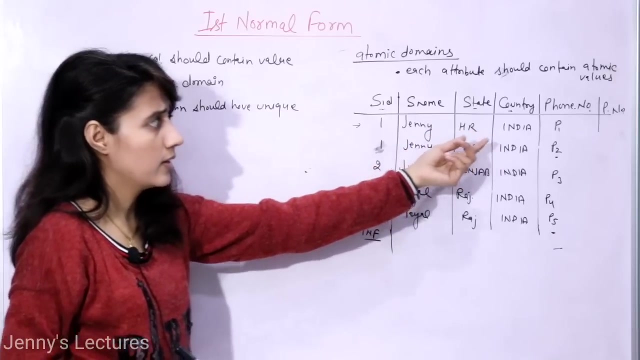 have unique name. it's not like that. here also I'm taking phone number and here also I'm taking phone number. if two columns are having same name, that is not correct. if this is the case, then that that table is not in first normal form- right, because obviously that would be incorrect. we will not able to find. 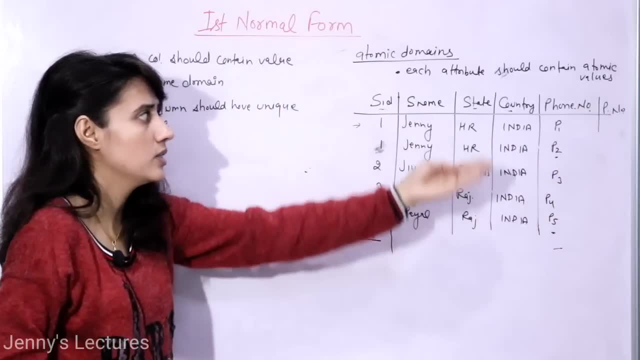 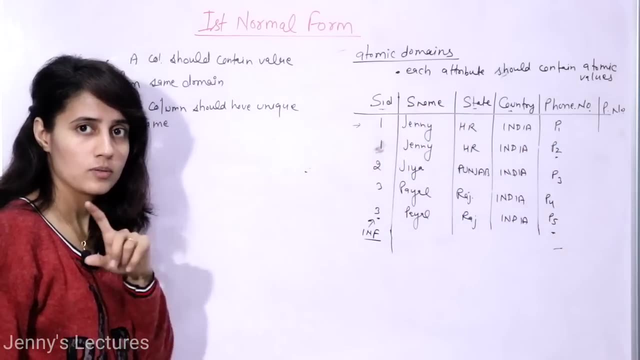 out which phone number we are asking. if someone is asking, then which phone number he is asking. right? this phone number or this phone number? right? if suppose I'm taking S name? S name. that is also not possible, right? so each column should have a unique name. that is third rule. 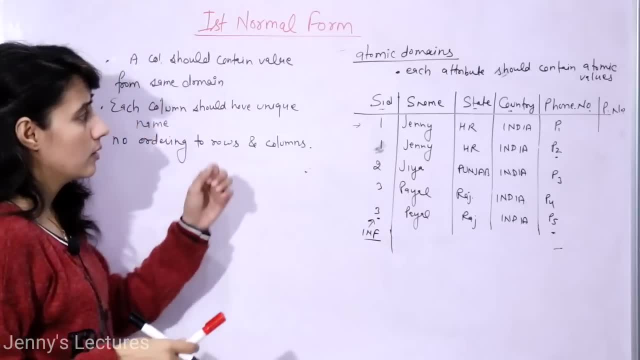 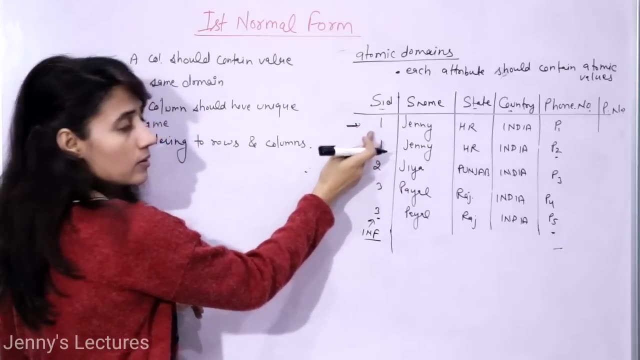 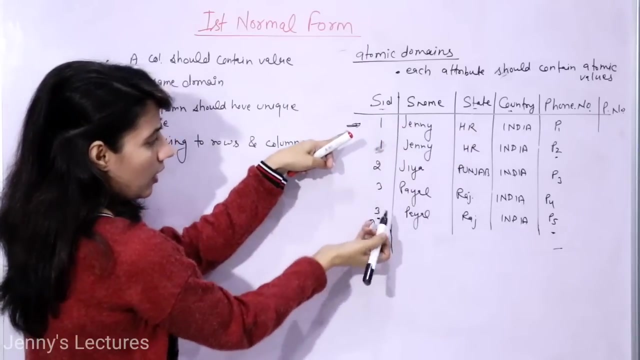 fine. fourth rule is what? no ordering to the rows and columns are applicable. see, it's not like that. this row you will will be first. this row would be second. no, maybe you can write one: Jenny, HR this information here. after that you can write this information three: Payal, Rajasthan, India and v5. 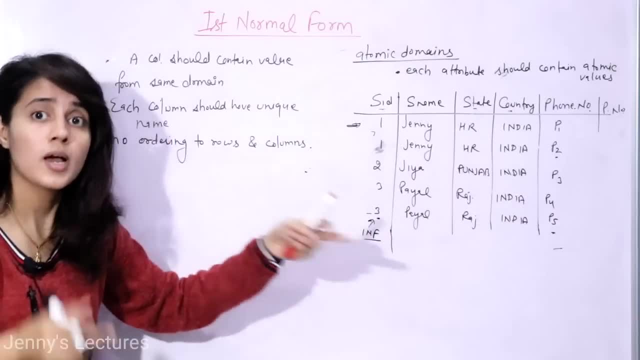 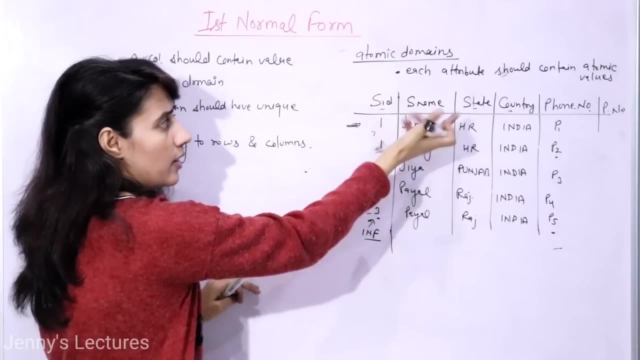 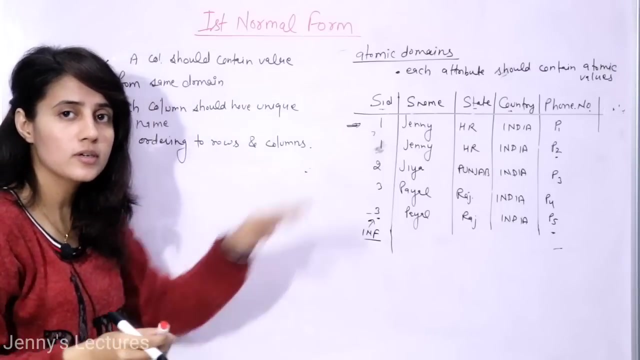 right. so no top to down ordering to the rows and no left to right ordering to the columns. maybe you can write this attribute here: SID, after that, maybe you can write SID after, after phone number. maybe you can write country here, state here. so the ordering does not matter. this is the fourth rule. fifth rule is no duplicate. 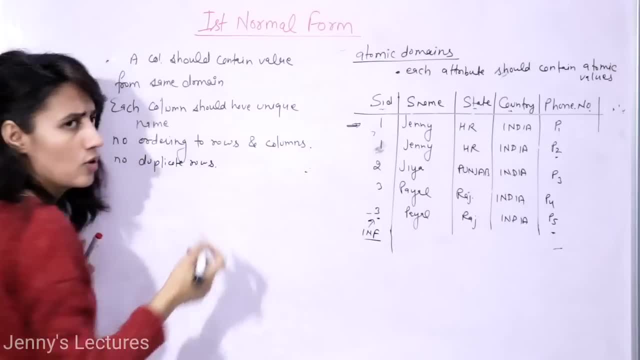 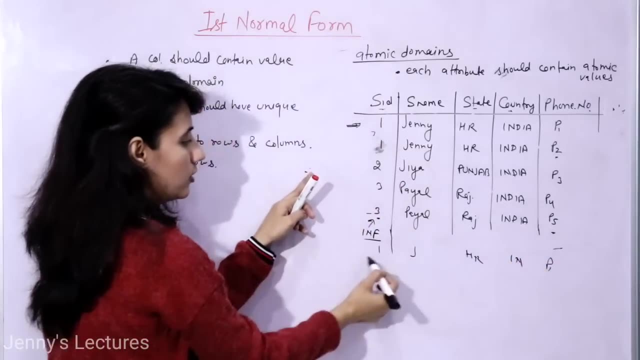 rows would be there. obviously it's not like that. here also, I'm storing one: Jenny, HR India and P1. this row and this row would be exactly same. so that cannot be a case. so that cannot be a case. so that cannot be a case. 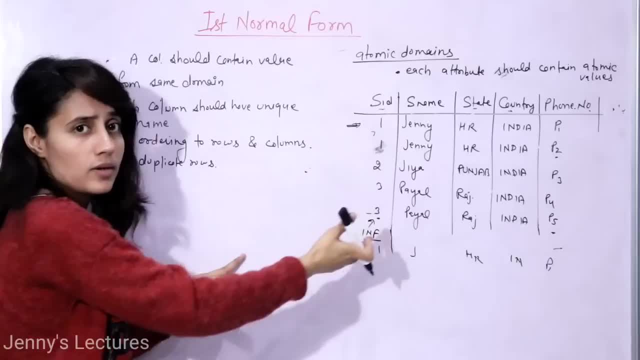 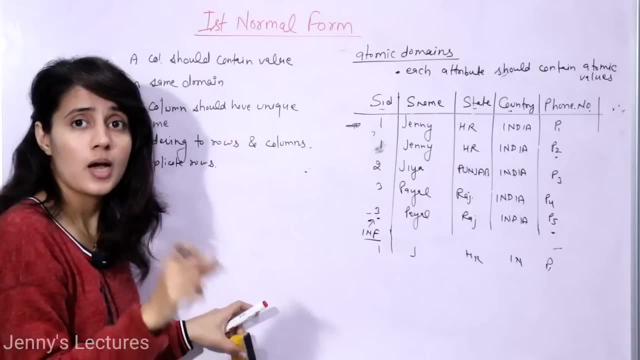 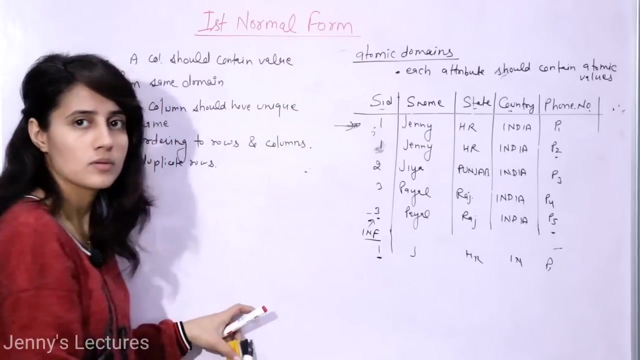 here and if, obviously, if we are taking one as a primary key, then this is not allowed and every relation or every table must have a primary key. and if, obviously, this relation is having a primary key, then this condition- it will not be a case here- will not occur right. so now, if every relation must, 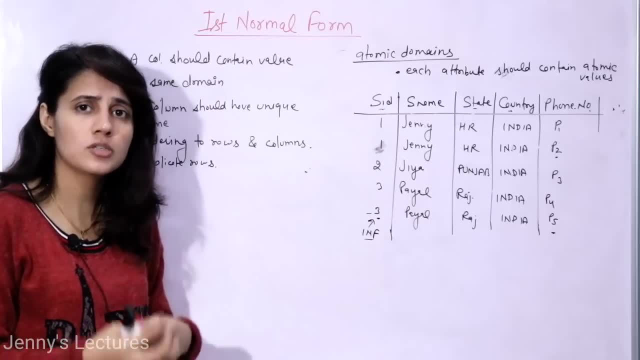 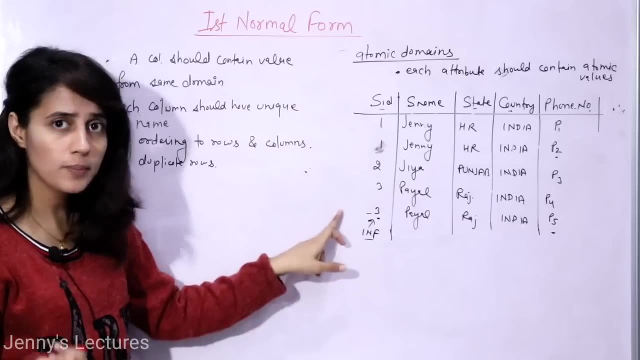 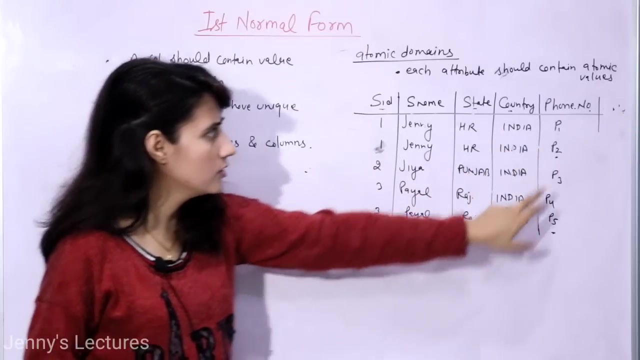 have a primary key. obviously, when you are designing a database and every relation must have table must have a primary key. so which is the primary key in this relation? SID cannot be a primary key because values are repeating here. such them also state also country also. but here in this case suppose I am taking only these entries. so 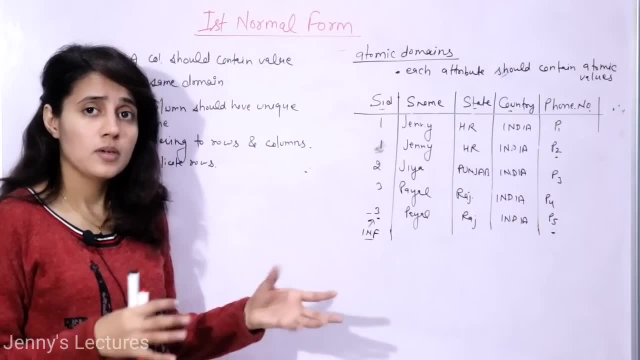 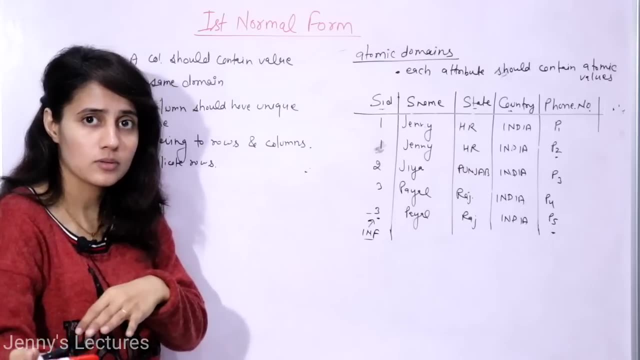 phone number you can consider as primary key. but? but sometimes it happens that you have a lot, maybe old SIM that you don't use and now that number has been assigned to another person, right? so maybe here also in the database I have here P1 and P1- same fair right. 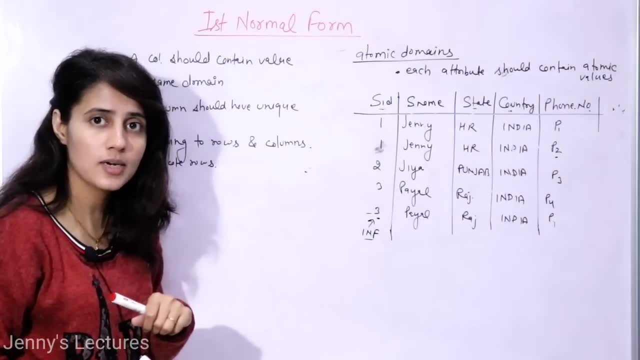 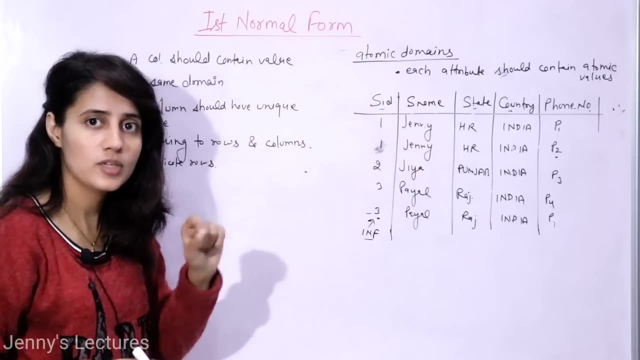 same phone number. in that case, what can be the primary key in this relation? it is not compulsory that primary key will contain only single attribute. we have already discussed all the type of keys in detail, right, you can check out that video in the side button. so now, here we can. 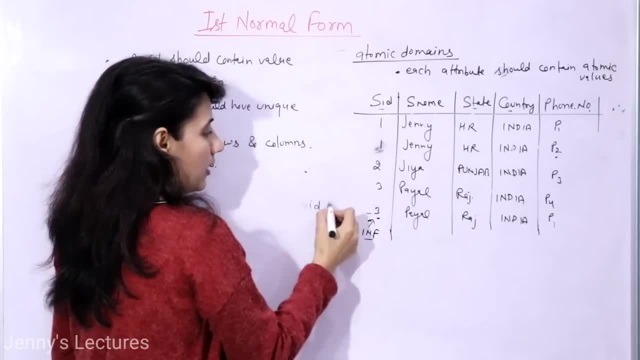 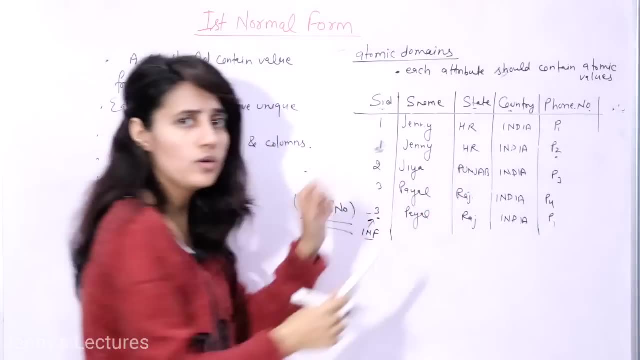 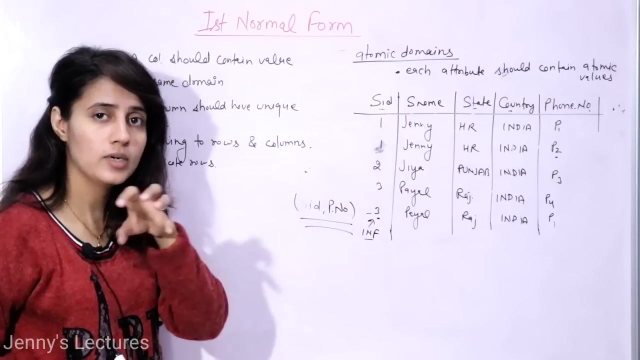 consider what- both sid and phone number- as a primary key right, because, as you can see, if you combine both sid and phone number, that will definitely uniquely identify each record in this tuple. i'm not going to, you know, going into the detail of primary key because we have already. 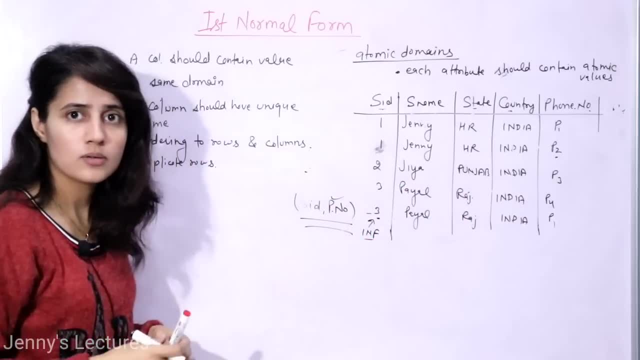 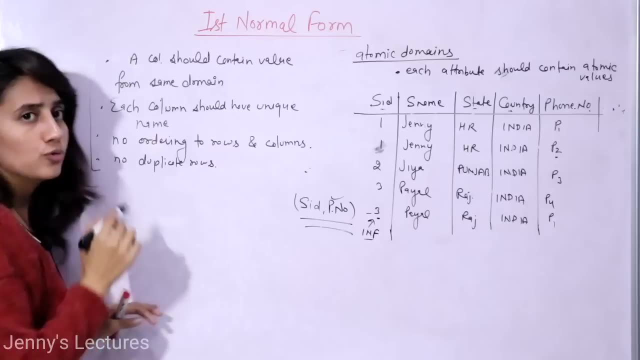 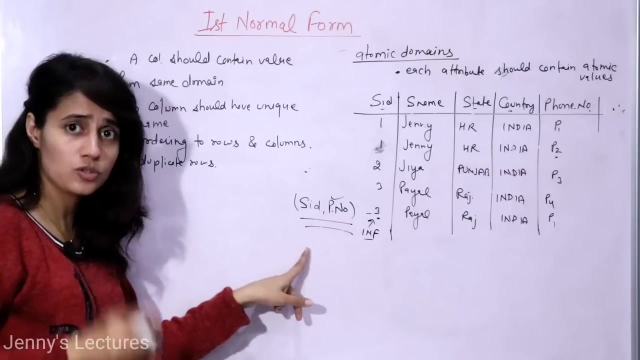 discussed in detail. so now this would be primary key in this relation. no problem, it is not compulsory that only sid must be a primary key. so now these are mainly four rules. a relation is in first normal form it if it will follow these rules right. otherwise it is not in first normal form. 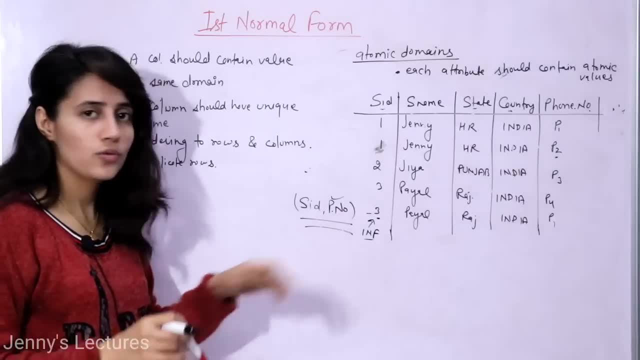 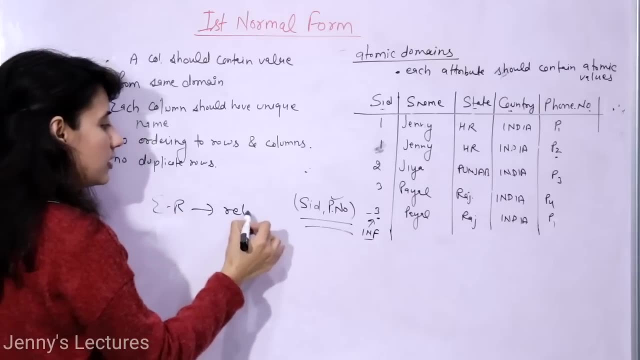 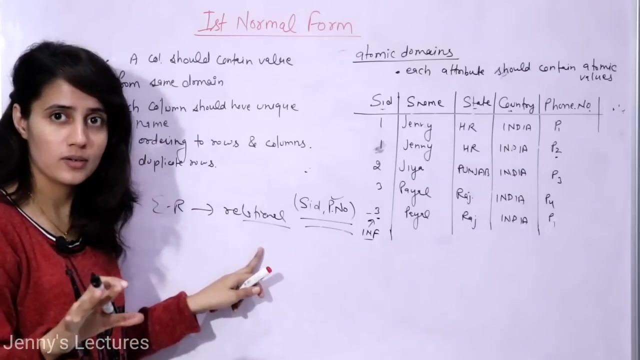 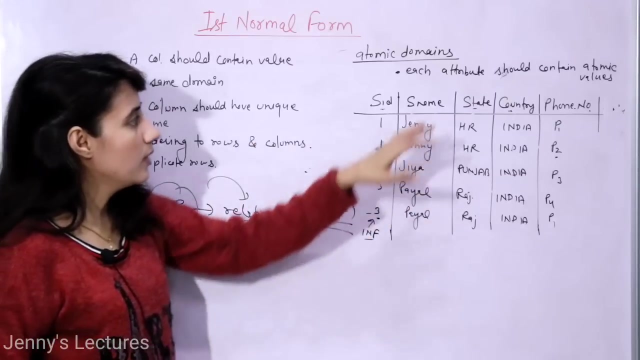 now the very important point is what this is. what a theoretical concept. first normal form. when er diagram is converted into relational schema, then definitely that schema would be in first normal form by default, right? definitely, when you are converting er diagram into relational schema, then every multi-valued attribute would contain a separate table. it's not like that. we will combine into the. 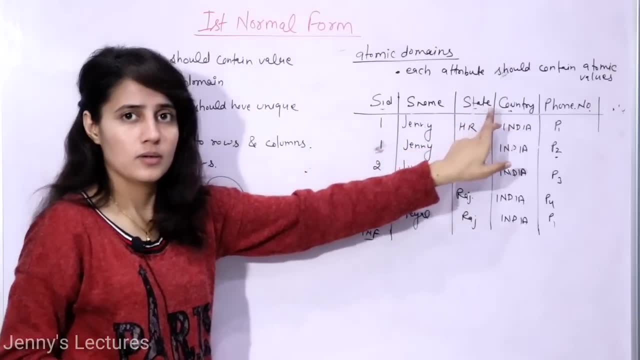 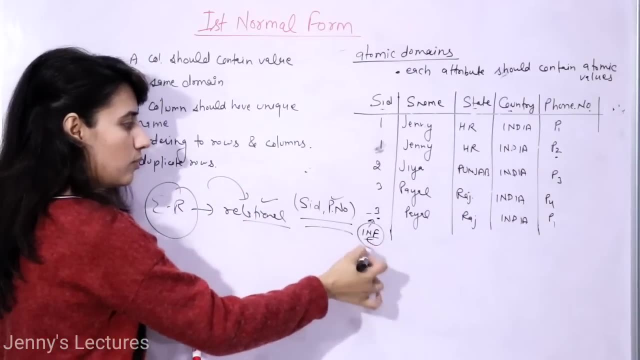 same table. right composite attribute- right composite attribute- would contain a separate table. it's not like that. we will combine. it would be denoted like this: with separate columns: right. so by default that would be in first normal form. now it's your responsibility to convert into second, third or bcnf, whatever you want. 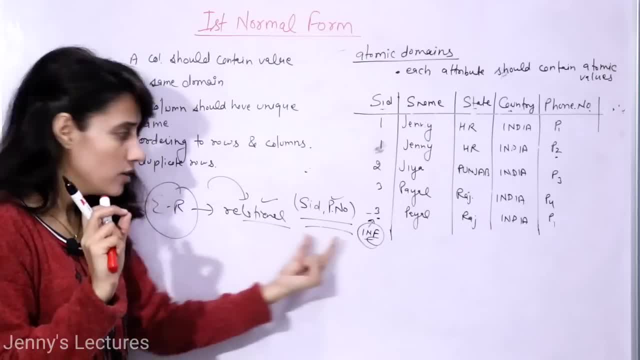 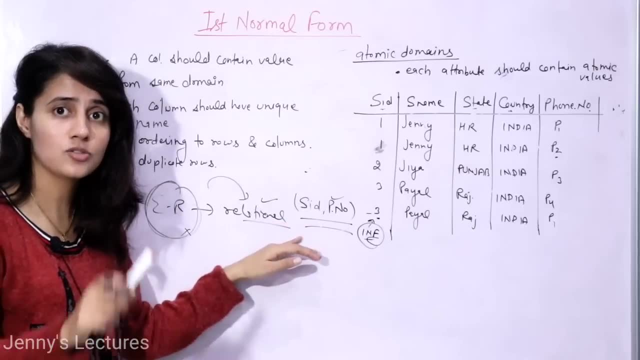 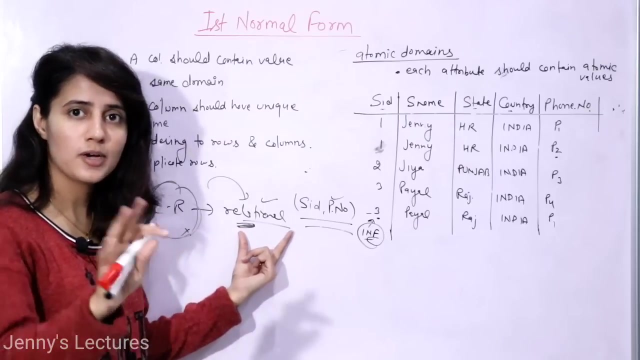 right. if this relational schema is not in first normal form, then definitely your er diagram is not good. or you can say your database design is not good, so you can say a good er design. design means good relational schema, you will get right. if bad er diagram is there, then definitely you will. 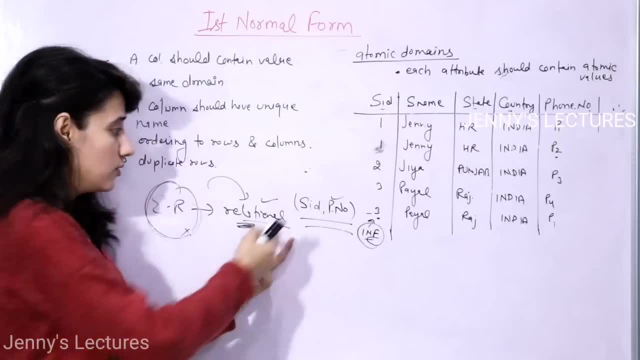 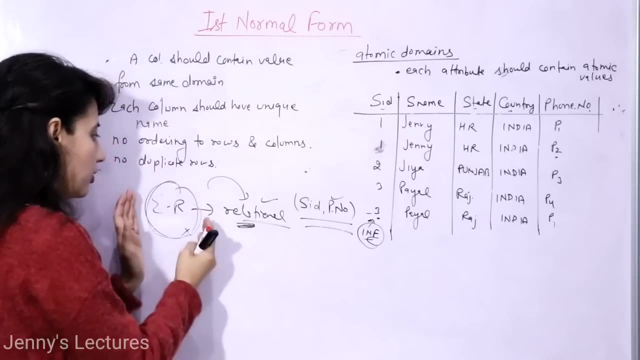 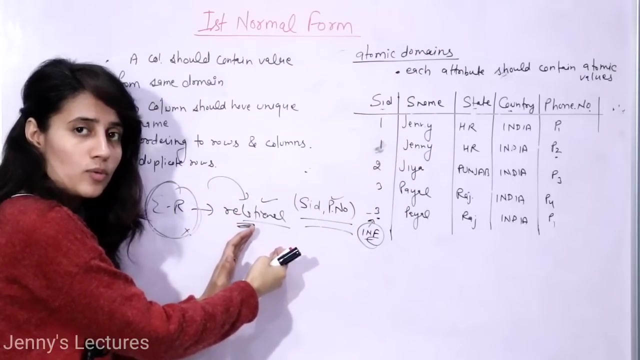 get a bad database design, fine. and if this generated relational schema is not in the desired normal form, then you can correct it. you can fix that problem into this er diagram. only you can fix it, and after that again you can convert and you will get the desired normal form in this relational. 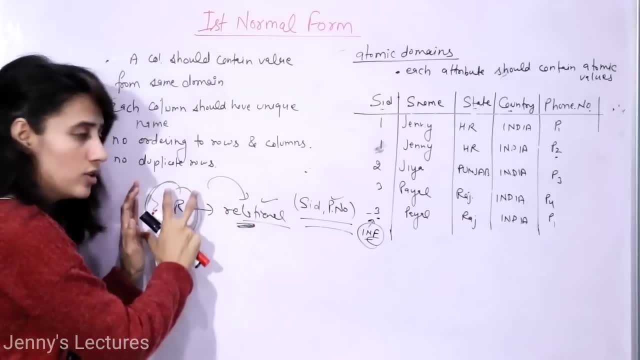 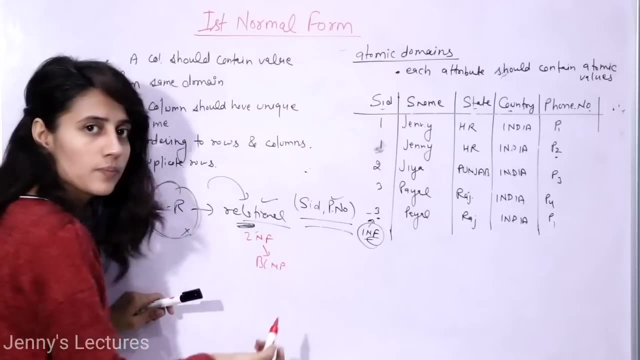 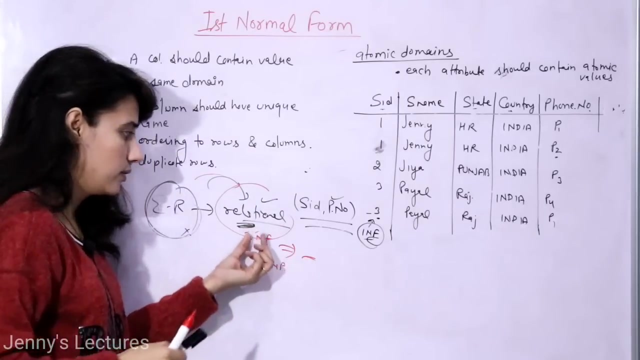 schema or, if you not fix the problem, into this er diagram. suppose this relational schema in a second normal form and i want that it should be in bcnf. then after converting into the relational schema i can apply somehow we will convert this thing from first normal form to second, third or bcnf. 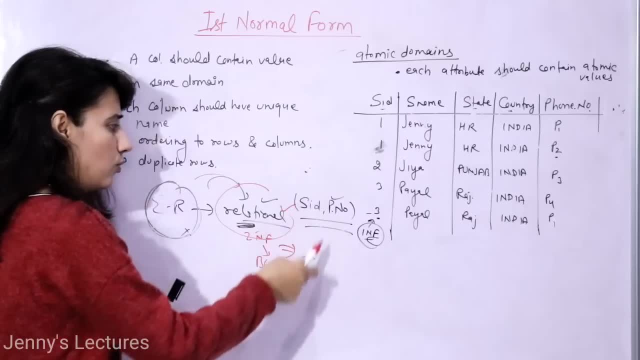 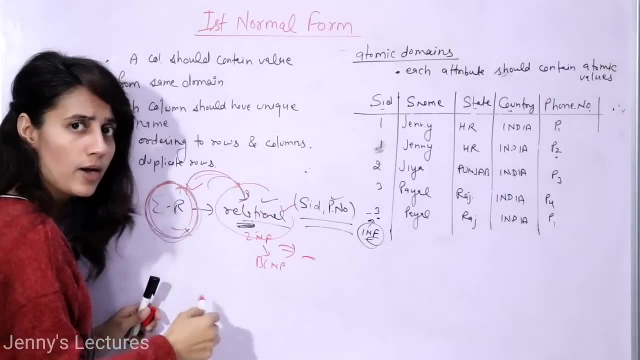 like this. that also we'll discuss in detail. so here also you can convert, or you can convert it into- you can fix this problem- into your er diagram also, and after that you can convert it into relational schema, and after that you will get that your relational schema is in bcnf right. so now here. 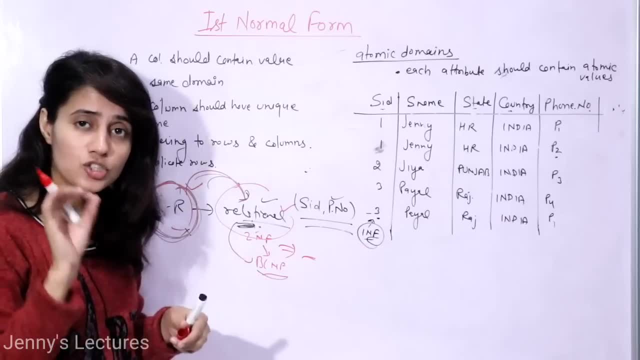 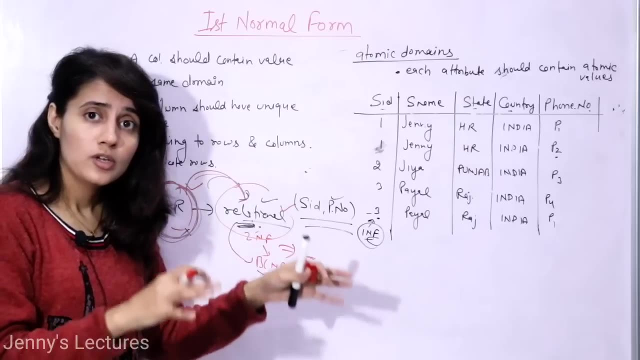 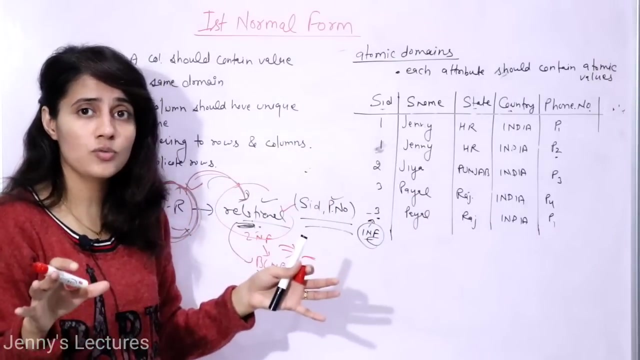 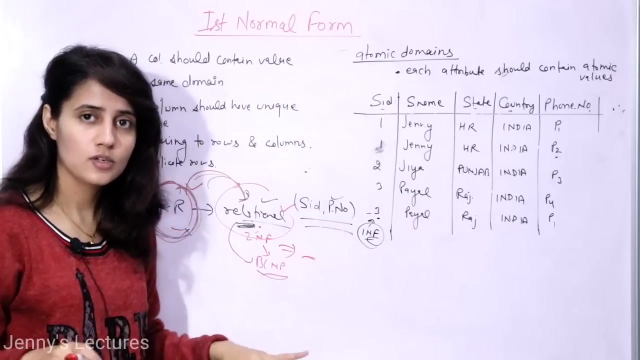 you can say first normal form is essential property of a relation in your relational schema, right, definitely your relational schema. if in a question it is given that consider this relational schema, then definitely that is in first normal form. they will never ask you in exam that the given relation is in first normal form or not. definitely it will be in first nf, right, so it is. 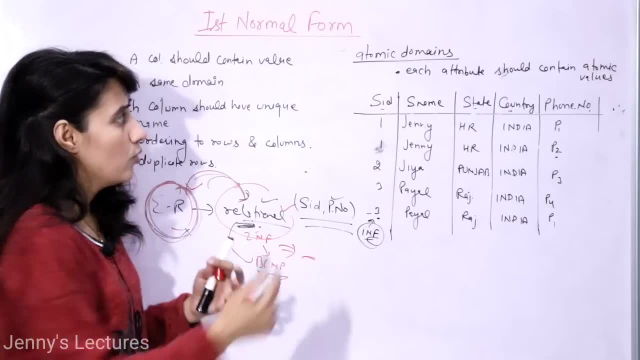 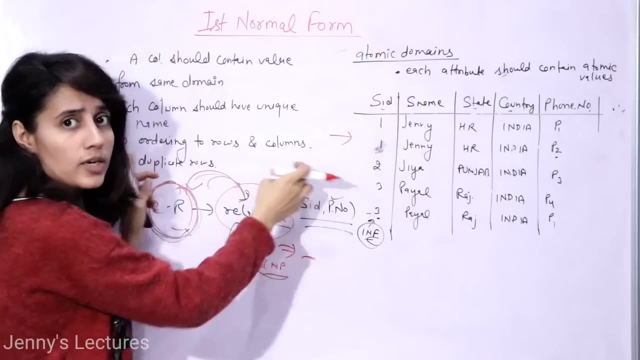 a theoretical concept now, different ways to convert. first way is this one. this is how we can convert that table into first normal form. second thing is what. you can divide the given table into two tables. i have told you that for each multi-valued attribute there would be a separate table. 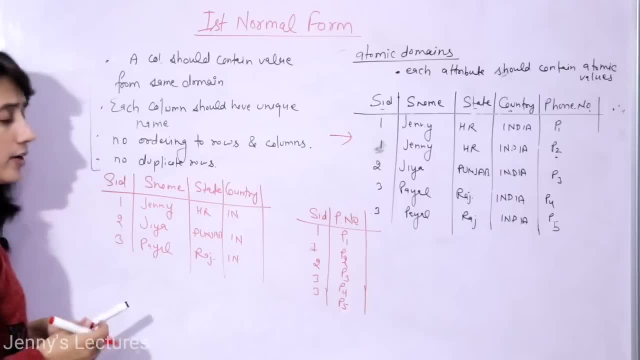 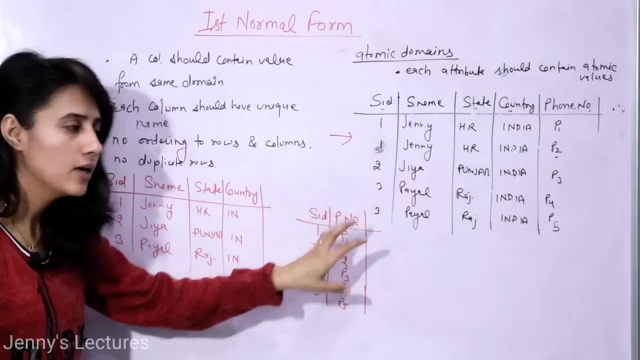 now, what is that second way? see? so this is the second way. you can divide the table into two tables. or you can say: for each multi-valued attribute you will create a separate table. so here i am taking that multi-valued attribute, that is phone number, and obviously with phone number i am taking 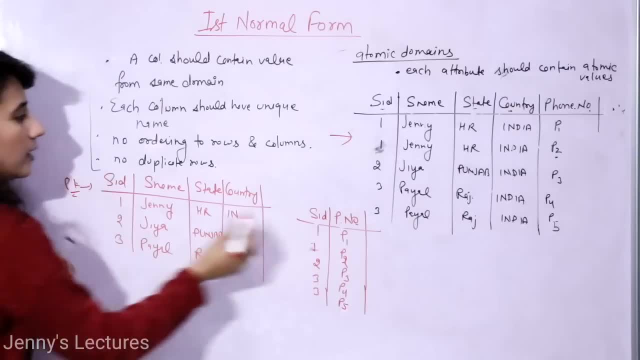 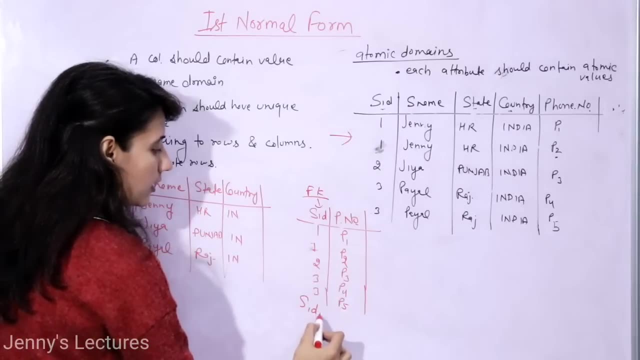 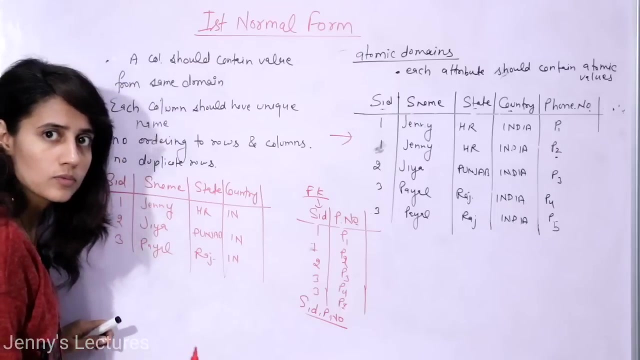 this one primary key. this is what primary key here in this table right- and here this will act as a foreign key right and for this table primary key would be what? both sid and phone number. if the situation is i am taking that this also p1 and this also p1. obviously, maybe we haven't. 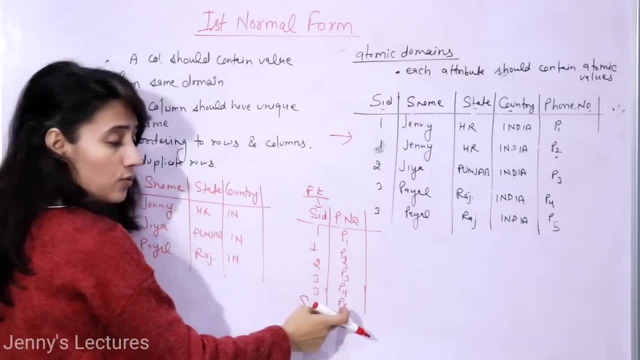 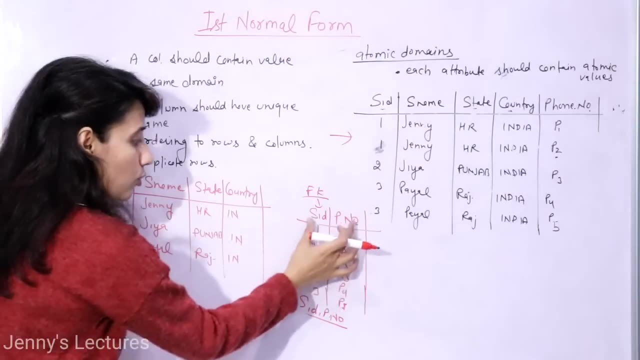 updated the old phone number of java and we haven't updated the old phone number of java, jenny, and that phone number has been assigned to another person now so that is also having p1, so we cannot take phone number as a primary key right. so now both would be primary key, here and this. 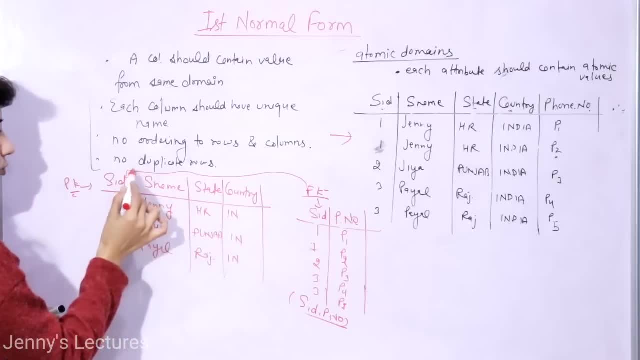 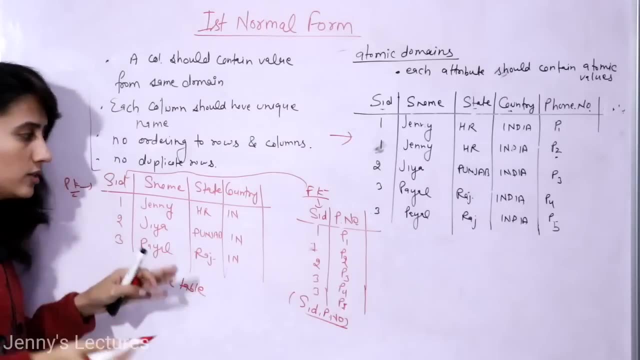 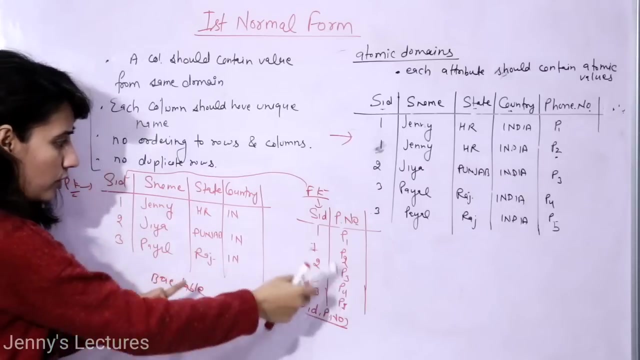 would act as a foreign key, so this would refer to this sid. this is our base table. now, right, so this is now. you can say: this is now in first normal form. these tables are in first normal form. all the conditions are satisfied. each cell is having only one value. each cell is having 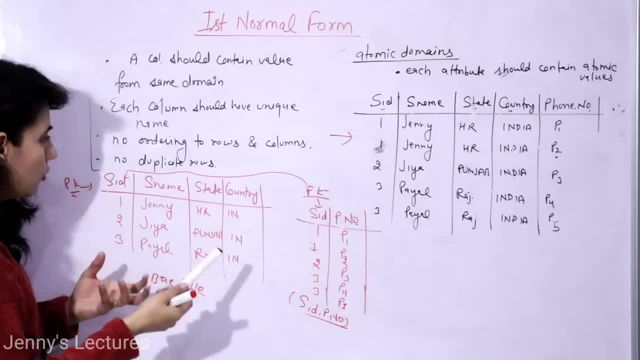 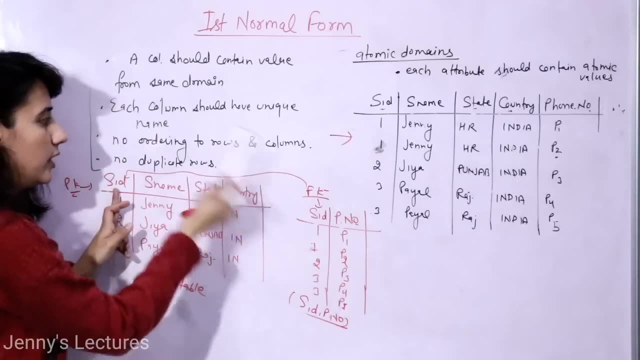 one value in that particular domain. right, and here also i am taking what: no duplicate rows are there. ordering of rows here also does not matter, and each column is having unique name. so these are in first normal form, right? this is how. this is the second way to convert a table into first normal. 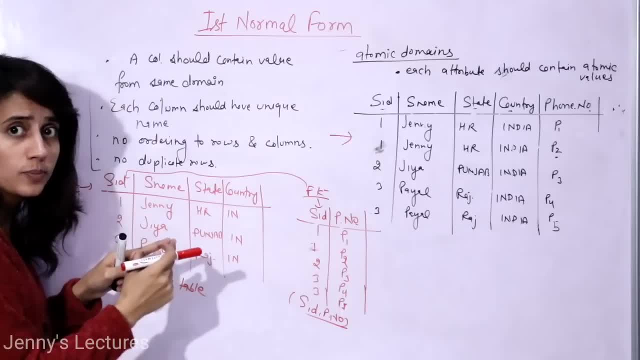 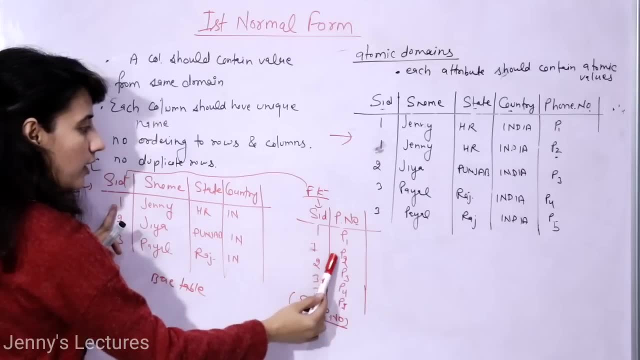 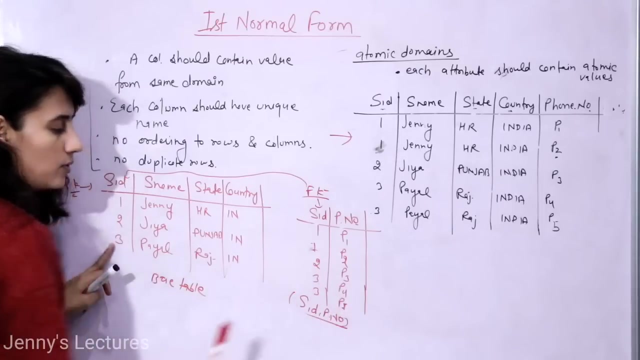 form right. see here: in this case one to many relationship are there, one sid is one, and this is in relationship with two phone numbers. means one to many p1 and p2 from here. one here i can get one and one here. three here i can get two rows, that is three and three, that is p4 and p5. so now, 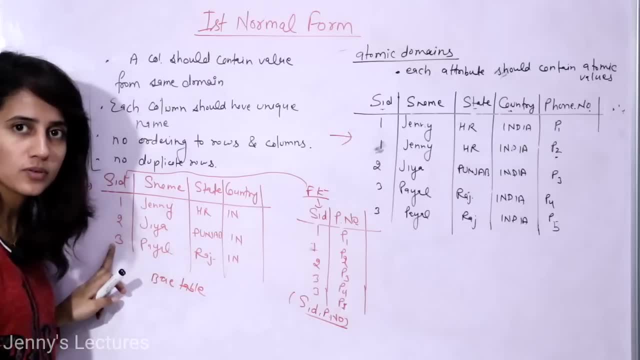 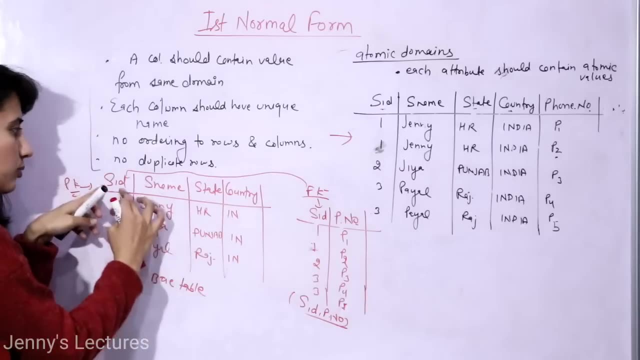 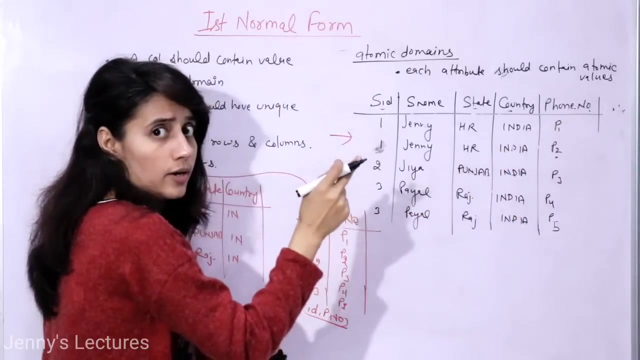 we know three pile is having two phone number, that is p4 and p5- right, because we have established a relation between these using foreign key, that is sid- right and this sid is primary in this relation. and third way is what you can take here we have multi, that multi-valued attribute, that is phone. 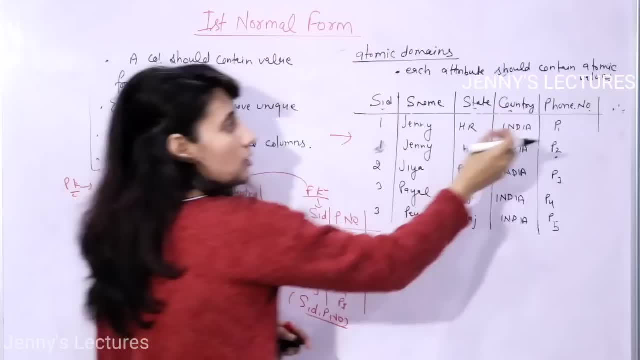 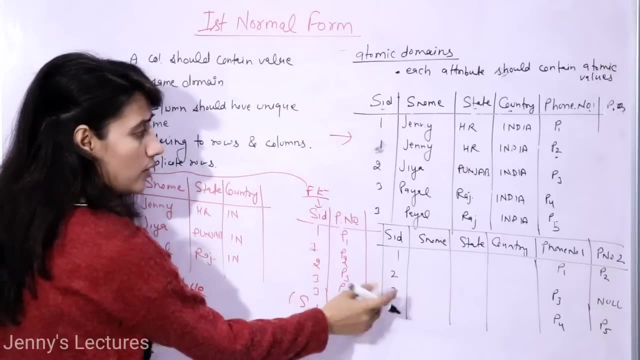 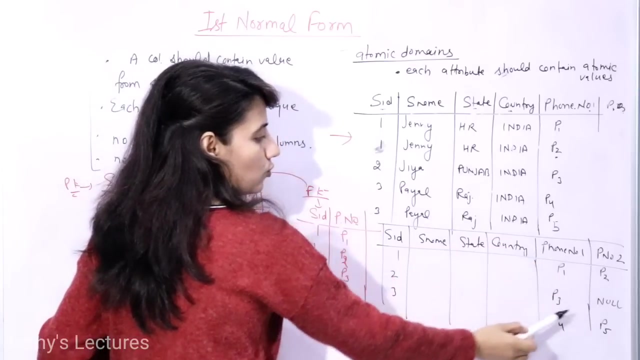 number. so in the same table you can do what? phone number one and phone number two, like this. so this is the third way here, what you have done. this multi-valued attribute we have divided into two columns, that is, phone number one and phone number two. so here i can write p1, p2, this 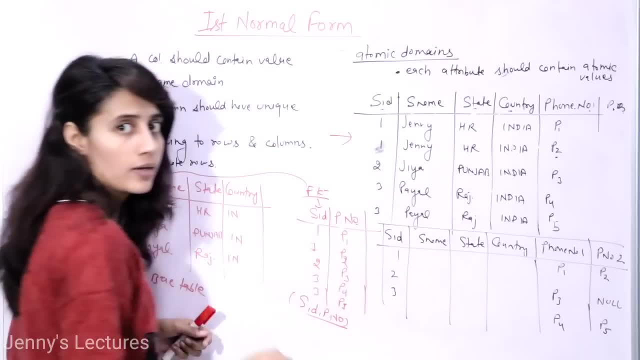 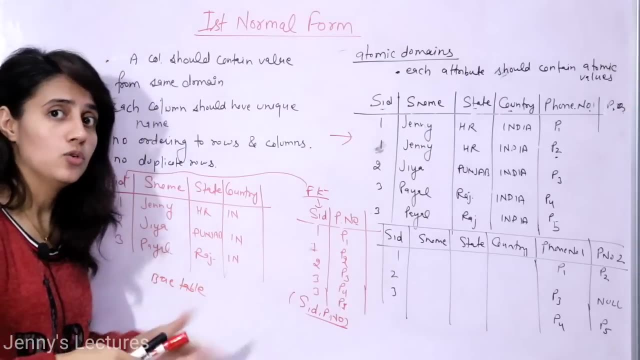 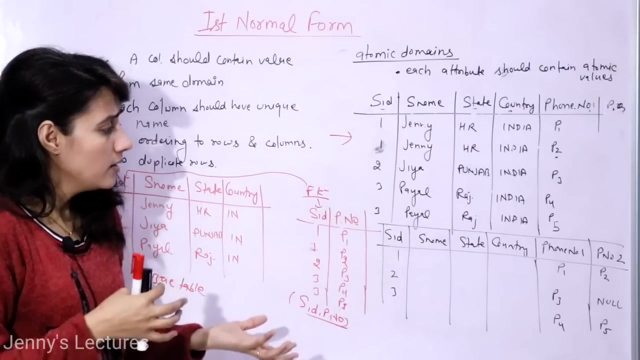 is having only p31 phone number, so this would be null here, not zero, it is null. and this is also having two phone number, that is, p4 and p5. but this is not a good way to convert it into first normal form, because almost this phone number is having the columns are having same name, right? we can't. 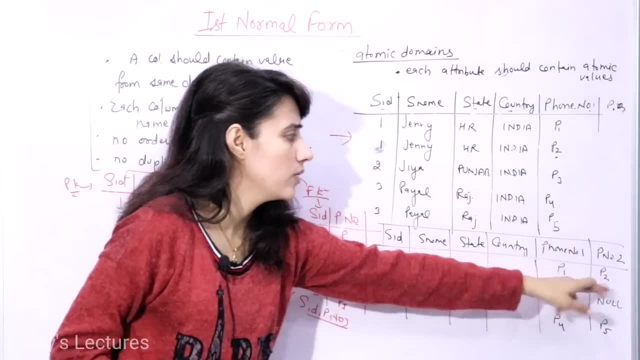 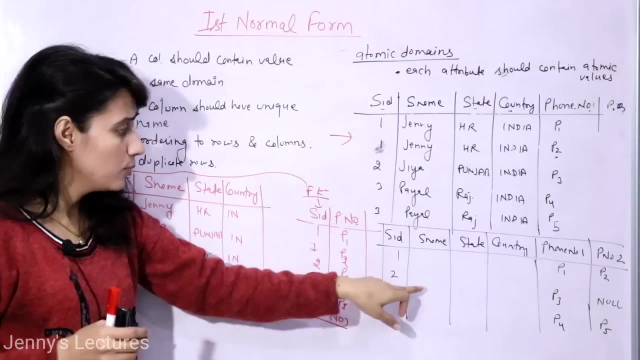 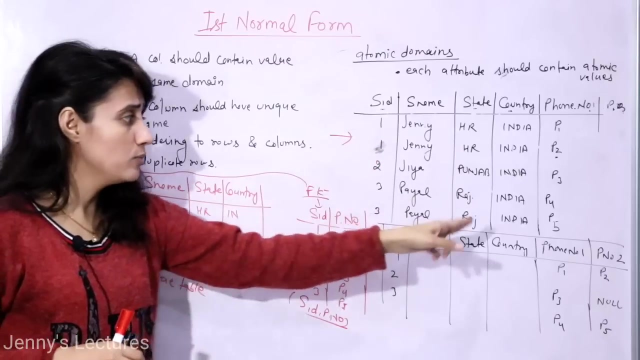 write p1 only in this case. so for example, if you write p1 and p2, in this case right in phone number one we will write p1, and in this phone number two we will write p2. maybe here also i can write p2, here i can write p1. so that would be ambiguous situation and here the problem again. one more: 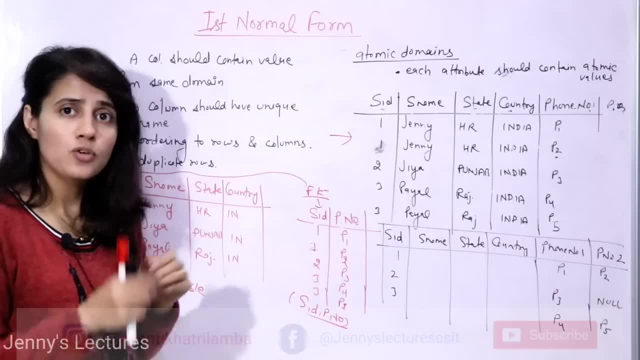 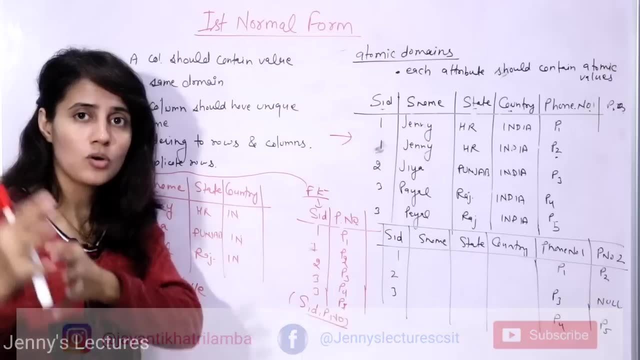 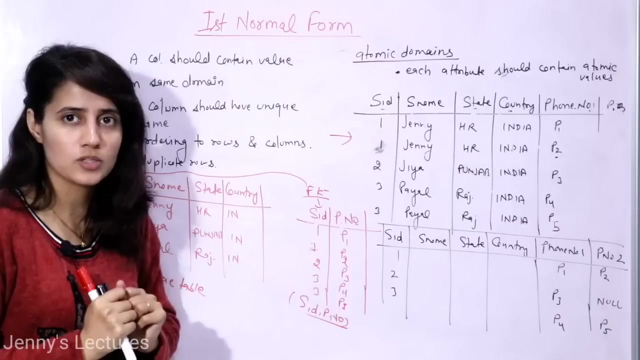 problem is what suppose phone number is. having one student is having 10 phone numbers, so 10 columns you have to make definitely right. and remaining students are having only one or two phone numbers, right? many nulls would be there in your table, so that is also a problematic situation, right? so this is. 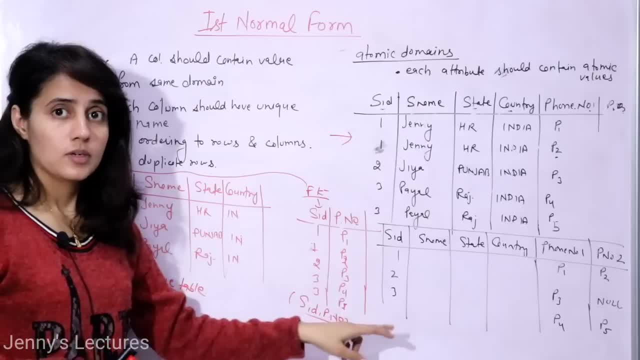 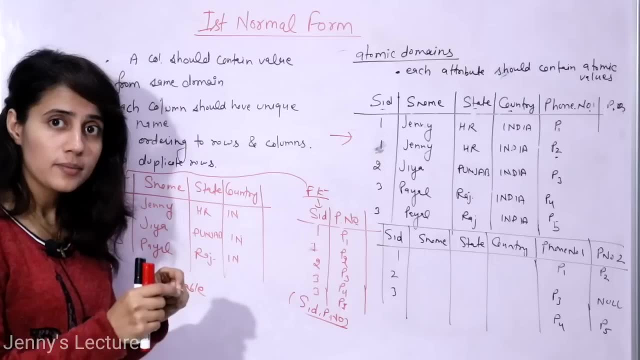 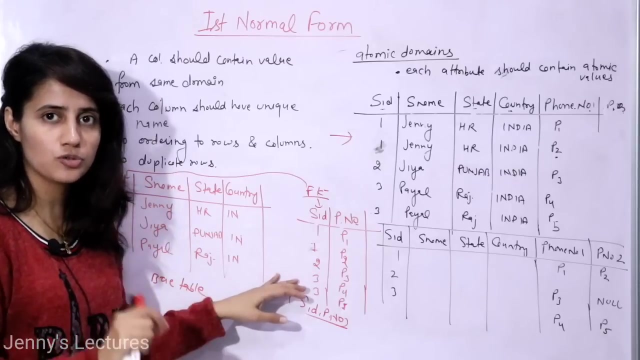 not a good idea to convert it like this. so here the best idea is just make a separate table for multi-valued attribute, right for composite attributes. make separate columns. fine, this is the best idea to convert a relation into first normal form right now. see, maybe you have a question. 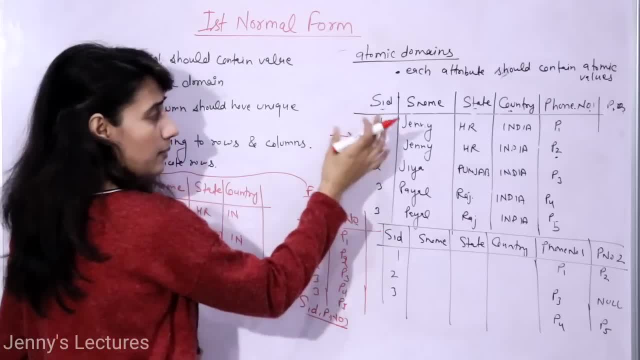 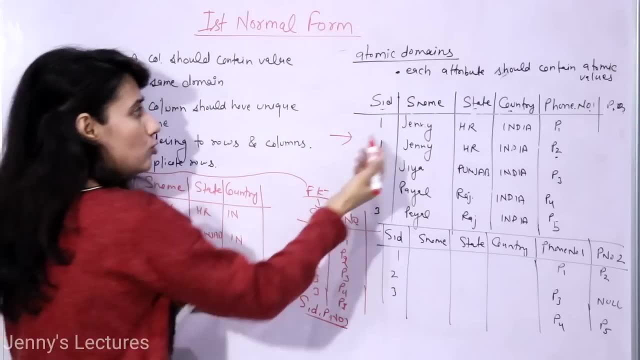 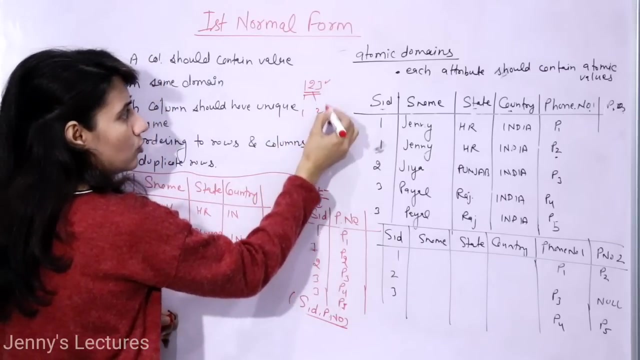 in your mind that if here I'm taking, I'm saying that all the columns should have atomic values, right, that cannot be decomposed further. so now, SIDs, I'm taking, suppose one, two, three. so now you will say that we can decompose it, like one, two and three, into three parts. so that is also what. 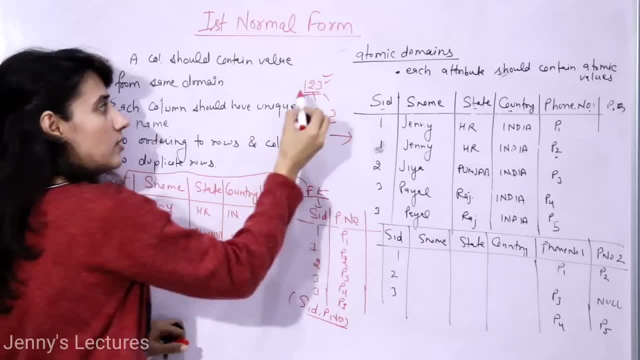 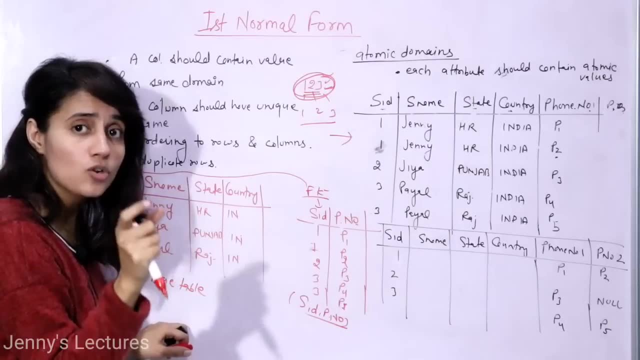 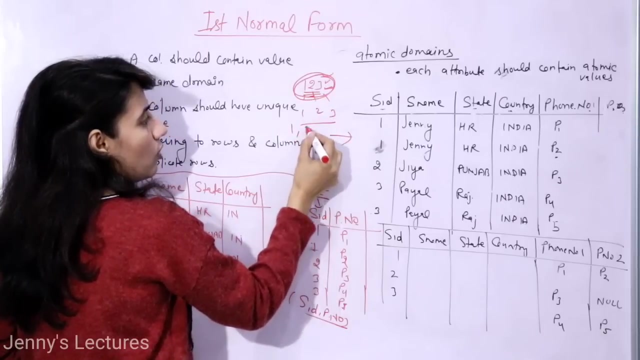 non-atomic. but the rule is what set this integers? integers are considered as atomic values, but set of integers is not containing atomic values. suppose I'm writing here, rather than one, two, three, I'm writing set one comma, two comma, three. this is not atomic. this can be further. 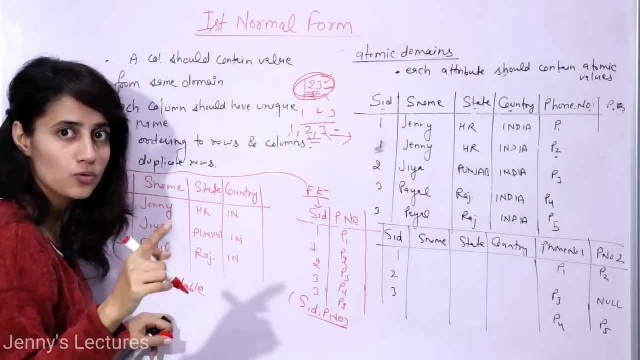 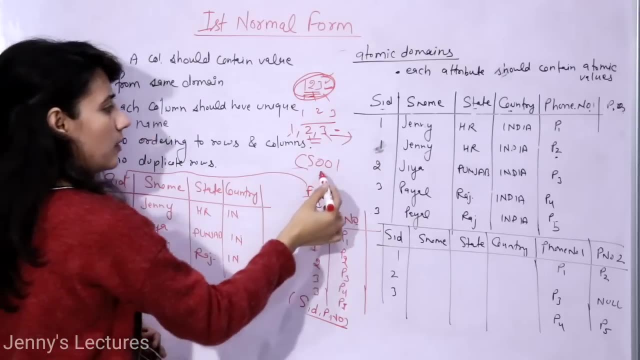 divided in one, two and three. this you need to take care right now. second is, what is now suppose employee ID? I am taking CS zero. zero one means CS is computer science department, and this is what idea for employee. so this is what non-atomic, this is not atomic right, because this can be. 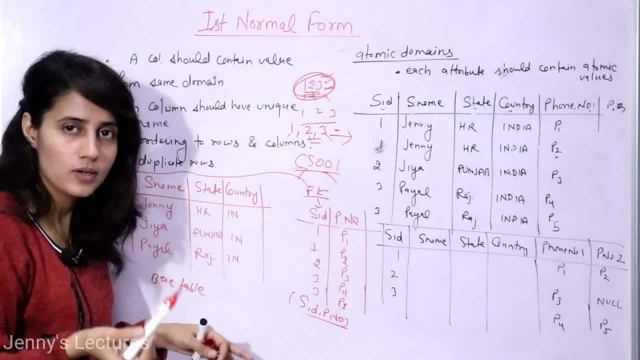 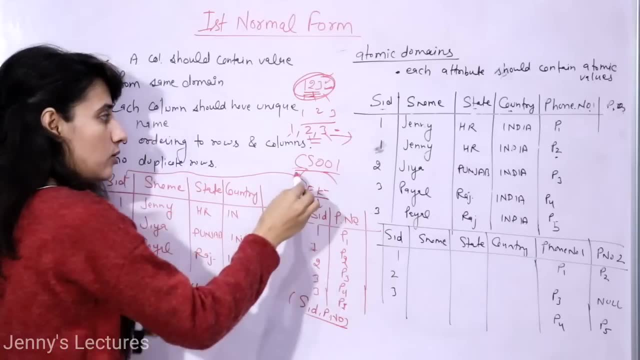 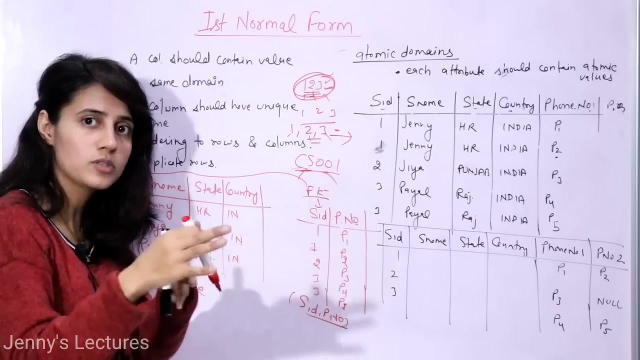 divided into CS and zero, zero one. fine so, and when? obviously when an employee will left one department and shift to another department, then you have to change this ID right. it cannot be CS if he has moved from CS to EE electrical department, so it should be EE. or you can say zero, zero one. 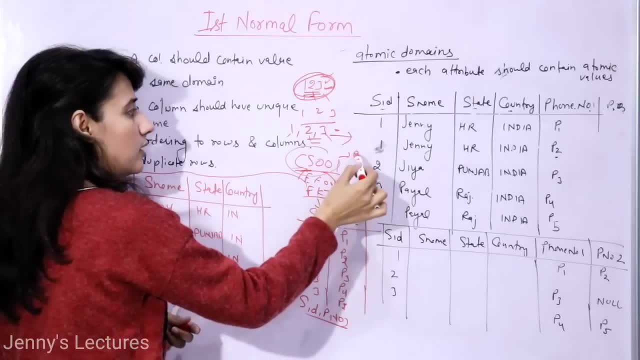 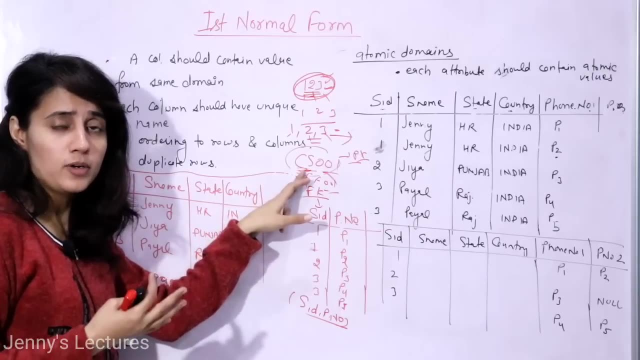 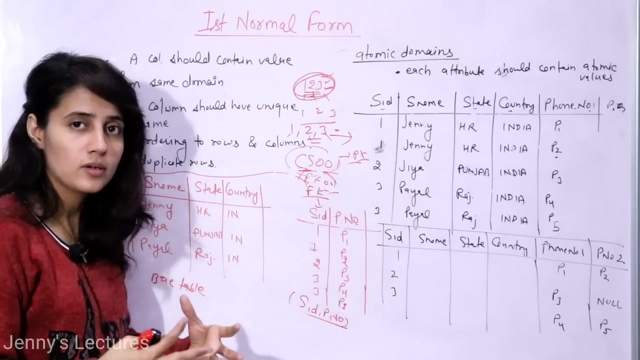 right. so if you take employee ID as a primary key in that situation, you will get some problem right. so now here to get the information about the department of the employee right. you know that the first two are the department, so you have to write down some coding and after that you will. 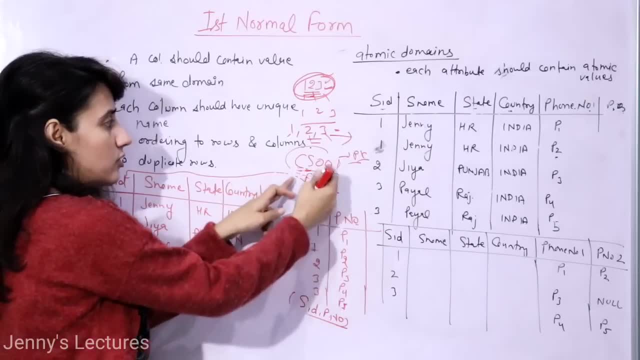 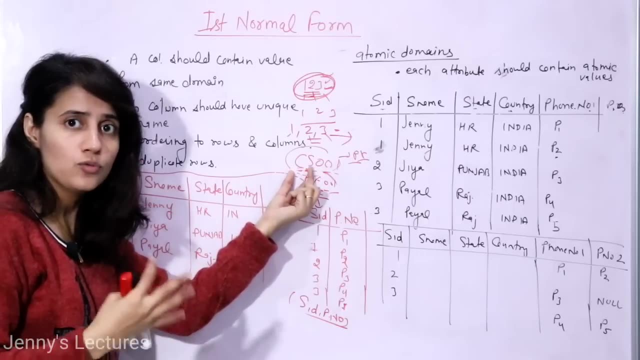 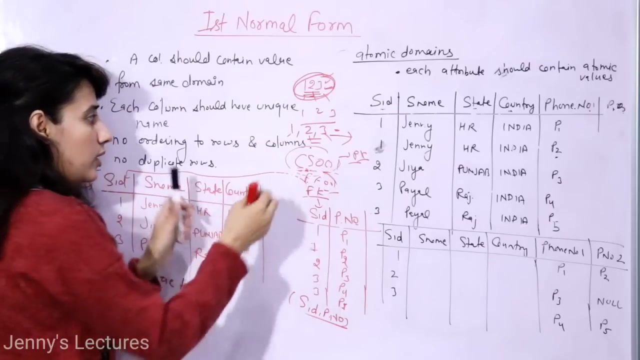 have to interpret this identifier like CS and zero zero one, and after that you will get what the department is: computer science, right so, but that encoding, that encoding would be in the application programs only, not in database. not in database. we are storing it like CS and zero zero one in database. we are storing employee ideas. complete this one, right, so this? 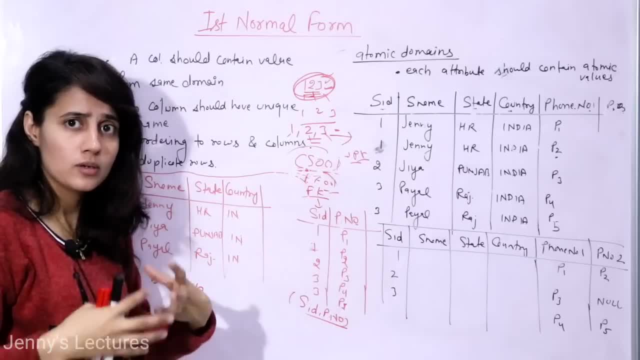 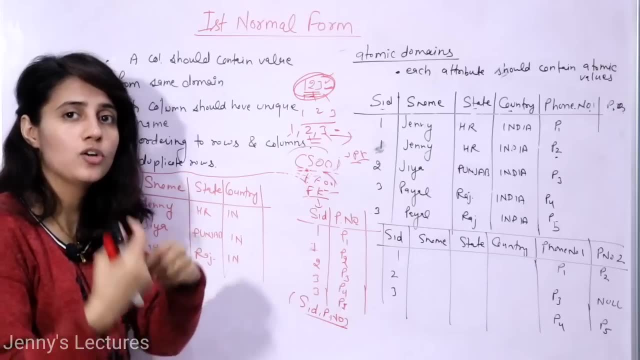 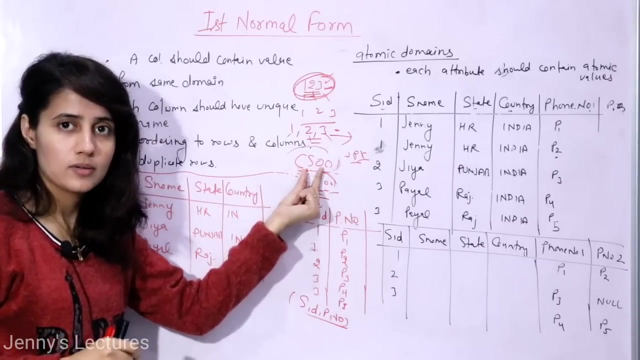 would be a problem. this would be non-atomic as far as we humans are using the system, right? but database application still treat it, as you can say, as atomic values. as long as it does not split this identifier, fine. as long as it doesn't require to split this identifier, then in that. 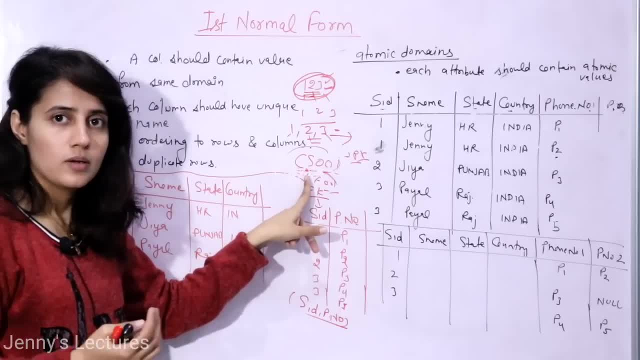 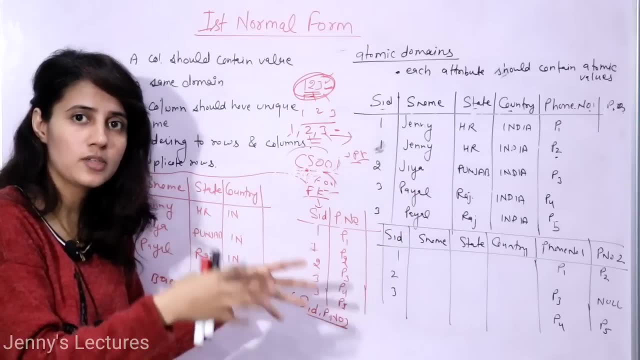 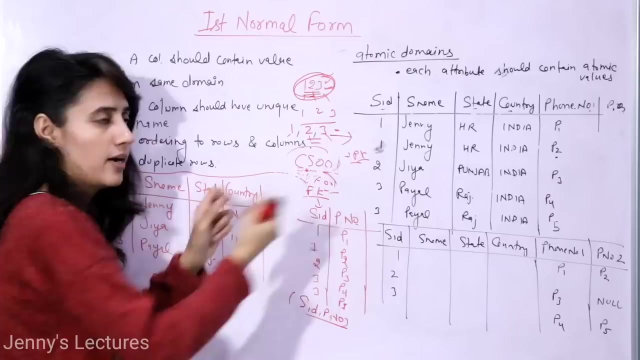 case you will consider it as an atomic value, because maybe in this relation, another attribute is there, that is of department. so using that attribute, that database application can get the information, that which is the department of the simple, rather than splitting, rather than interpreting this identifier right. so in that case still, the university schema would be in our 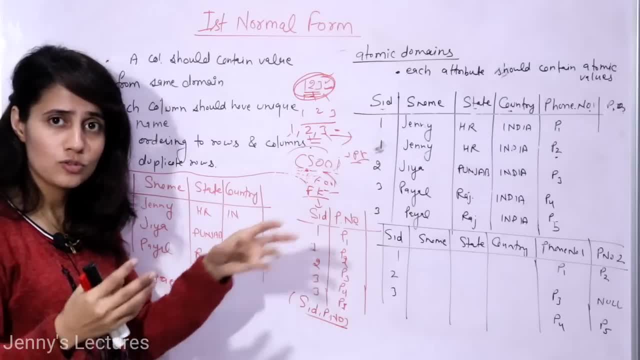 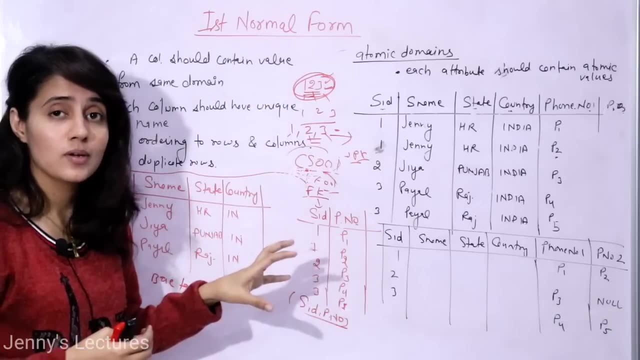 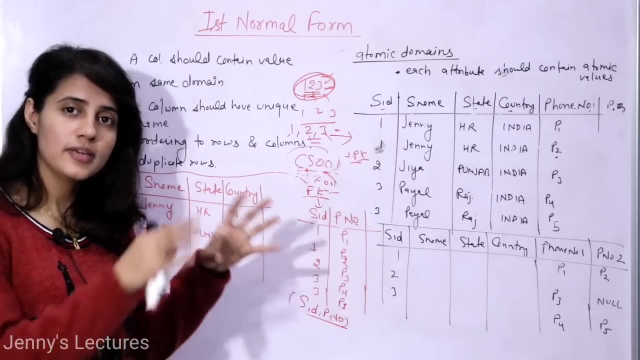 first normal form. so these points are those students who are very curious, right? these are extra points, not the basic whatever in the first normal form. right now. I hope I was able to clear your doubts, if you have these kind of doubts. so this is all about first normal form. in the next video we'll 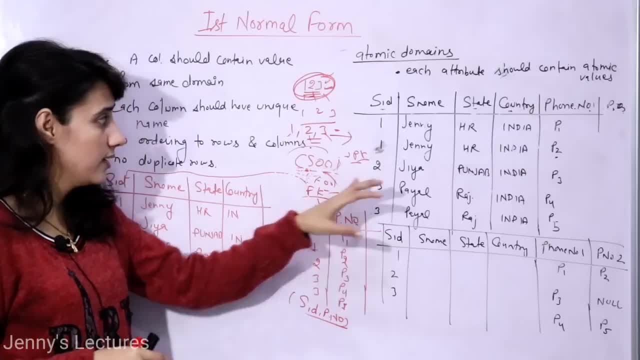 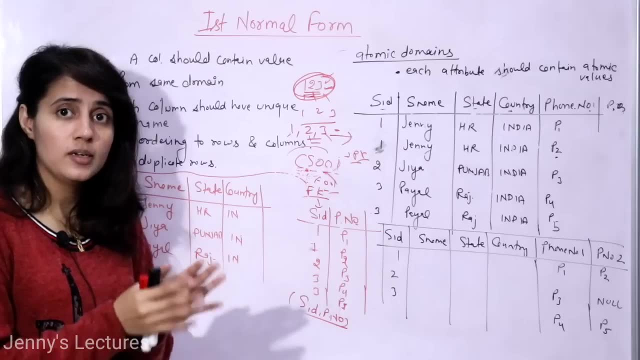 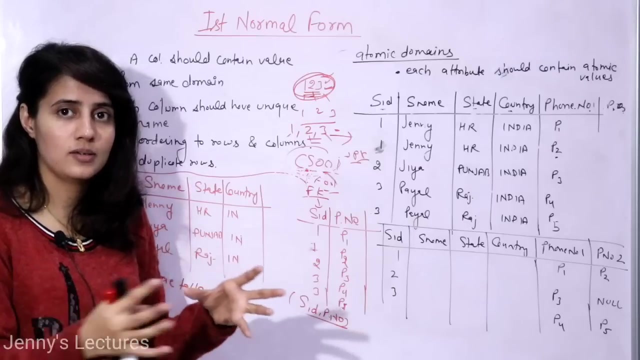 discuss what is second normal form and if a given relation is given, then how to identify that that particular relation is in second normal form or not, right? so basically, after that, after this video, in the next video, we will need all the these functional dependencies concept, and that keys. 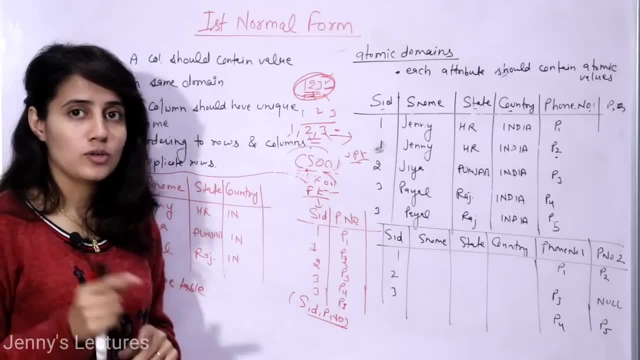 concept right. so you must revise that concept first of all. so now I'll see in the next video. till then, bye, bye, take care. So can you achieve a high salary in cybersecurity? Yes, Am I hating on those who have a six-figure income? No, There's a lot of hype regarding high-paying salaries in cybersecurity. If you look at cybersecurity training, clickbait titles, social media, you'll find that one marketing tool. 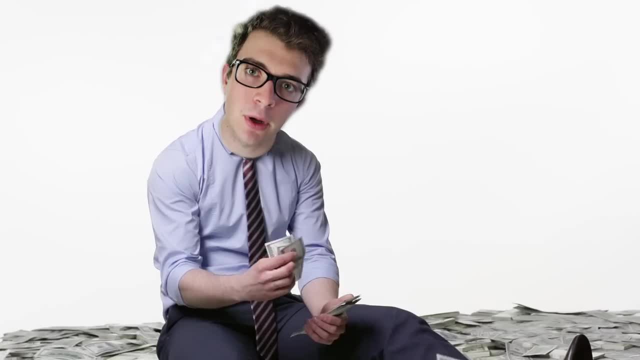 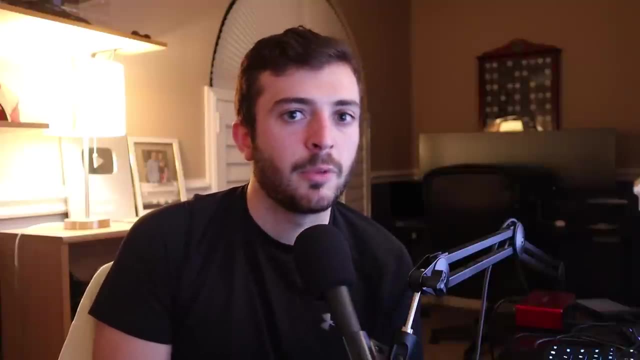 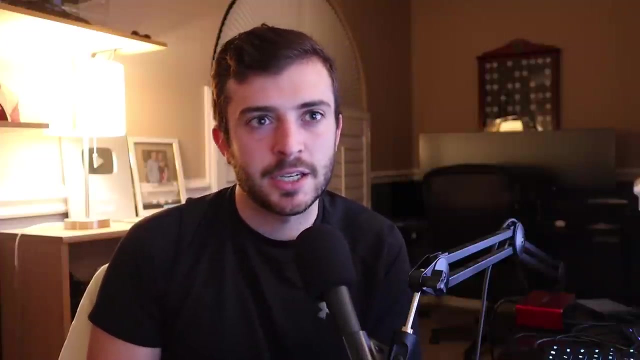 that these training programs universities use is the six-figure income salary or just high salaries in cybersecurity. There isn't anything necessarily inherently false about this statement. In fact I use it on my own course landing page, but it is not sort of a misconception in security. 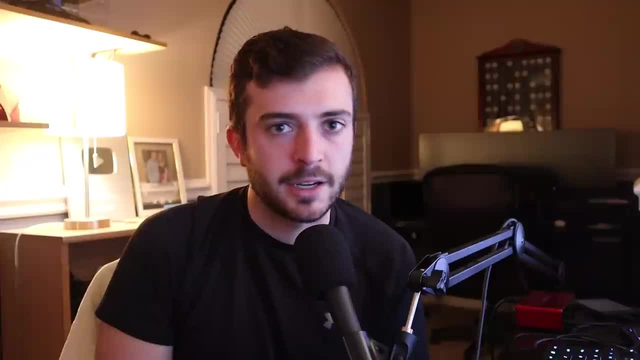 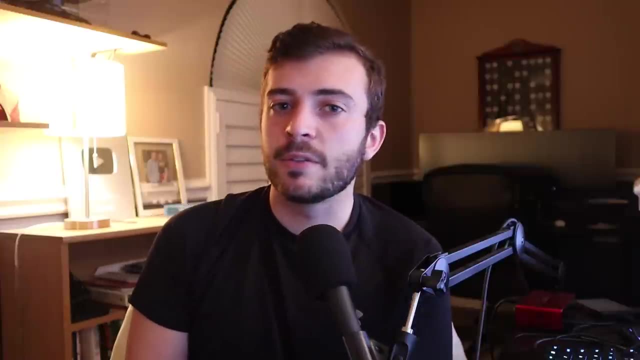 especially when you take a look at entry-level security jobs, a topic that I often talk about on this channel- You'll see that this isn't necessarily reality. So, yet again, another video on the reality of cybersecurity careers, and I'm probably stating a lot of the obvious in this. 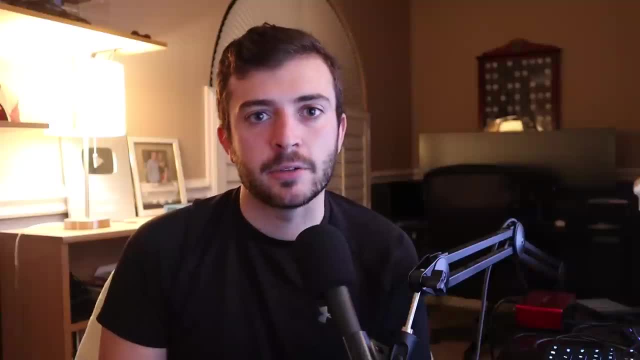 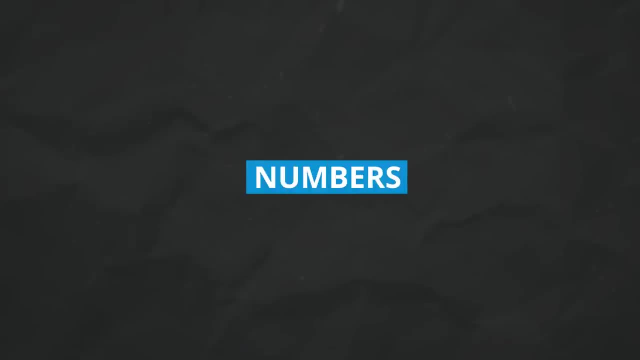 video, but I do want to take a look at high salaries in cybersecurity and why that's sort of a myth in cybersecurity. I'm going to take a look at high salaries in cybersecurity and why that's sort of a myth in this industry. I will start with numbers, or more specifically: the average cybersecurity salaries. Now, because I am from the United States and I'm most familiar with American economics, I'm going to be breaking everything down between the United States and dollars and looking at the actual individual states' breakdowns. So the six-figure income: 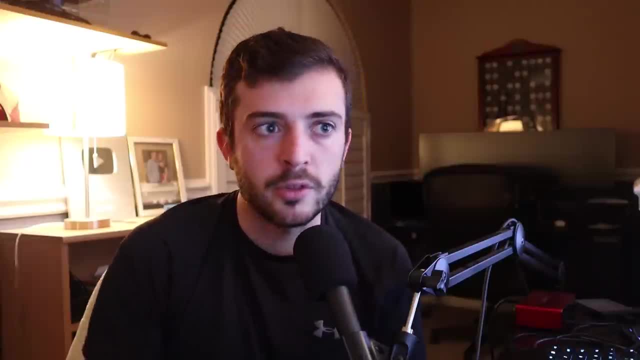 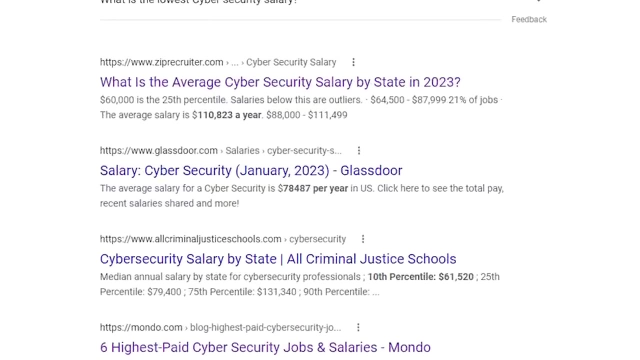 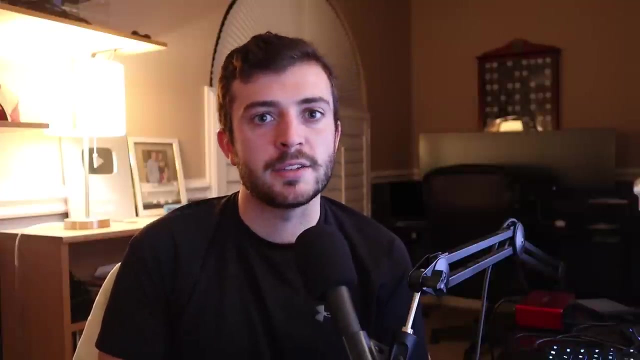 in cybersecurity. yes, that's awesome. If you Google the median salary of a cybersecurity professional or job, you're going to probably find something in the middle of the list, So that's great. But these numbers lack context in two ways in my opinion. So if you go on a website